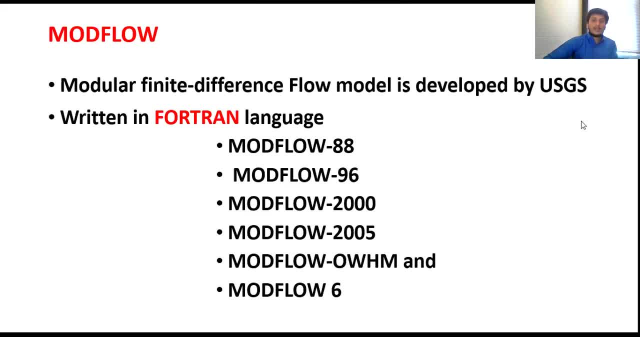 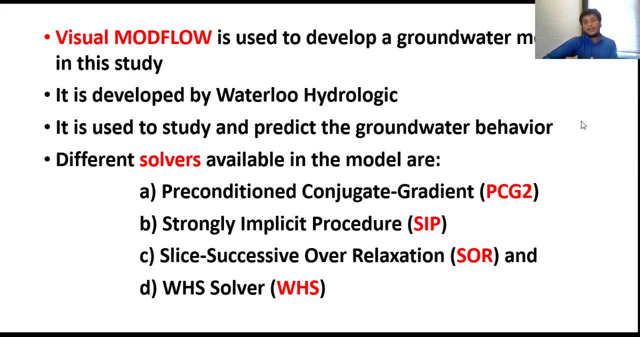 groundwater flow modeling in modflow. So going to visual modflow. visual modflow is available in 2D and 3D, So 2D, we want to see the 2D version. So visual modflow: it is like it is designed to model the groundwater. 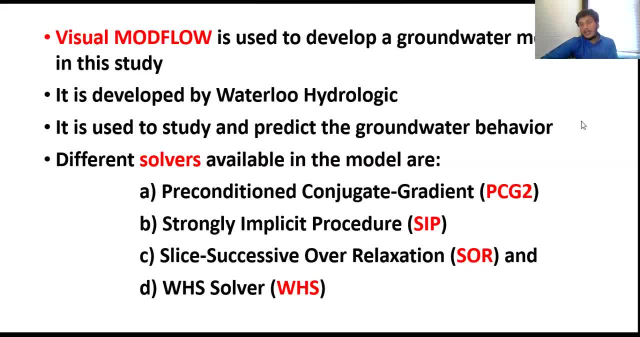 flow model and it is developed by. it was developed by Waterloo Hydrology Company. So these are different solvers available for, available in visual modflow. modflow solvers has like importance in modeling the getting the output. so in some conditions some solvers won't allow us to like they will. they will write it. 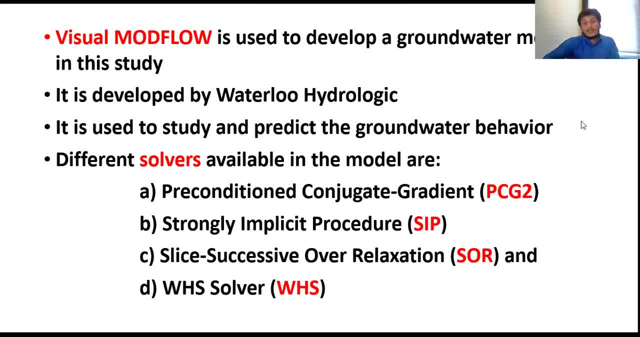 they will use, they will cause an error. so in certain situations we could, you could use, in those situations we can use the other solver. so here we can see like WHS solver, which is which is like which, if no other program run without any error, like if you got any error in any other other solvers, most probably WHS. 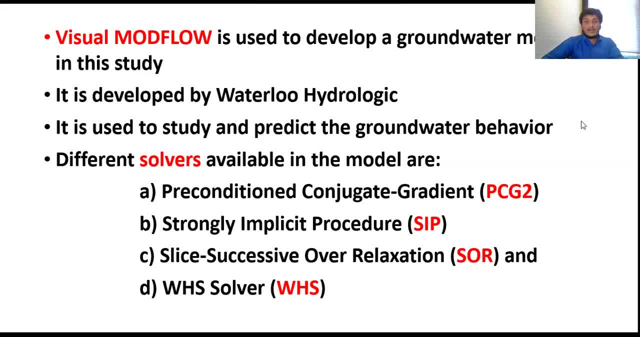 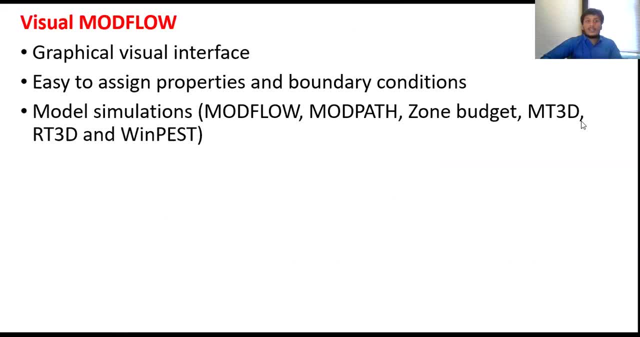 solver would help us in running a model and, yeah, in the visual modflow. these are the simulations available for the model modflow: modpath: zone budget. zone budget has it's like it, will you, it, will you, it? will you the total input to the aquifer or region, or? 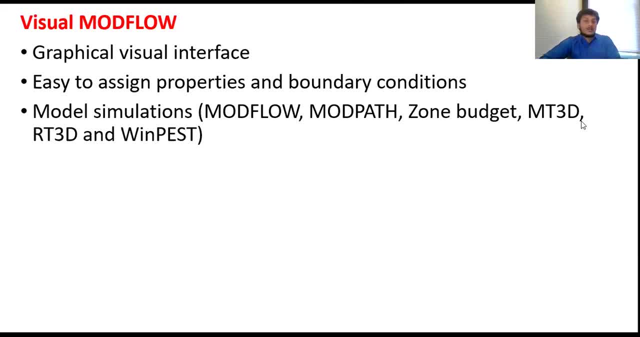 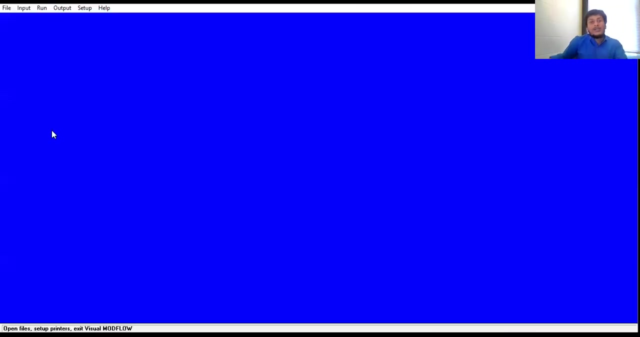 whatever. so so amount of water into the, into the floor surface or aquifer, and the water went outside from that. so it will give you kind of budgeting, water budgeting. and yeah, the graphical visual interface is the. is the uniqueness of the visual mod flow like good graphical visual interface, i don't say it's yeah. so coming to the software, so 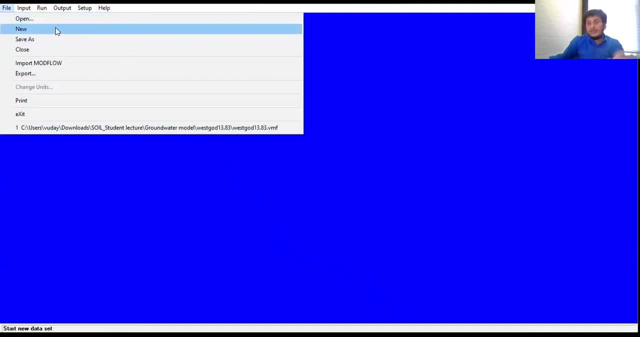 so this is a visual mod flow window, so we need to open the. if we have any existing files to edit or do we can open the existing file. so right now we'll. first i'll try to create a new file and view an overview on the on the on the visual mode flow. then i'll try to go back to the existing file. 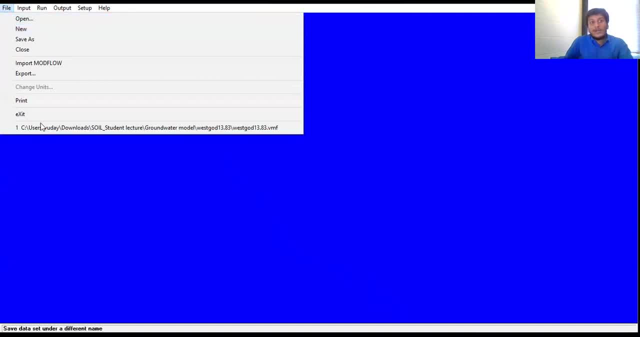 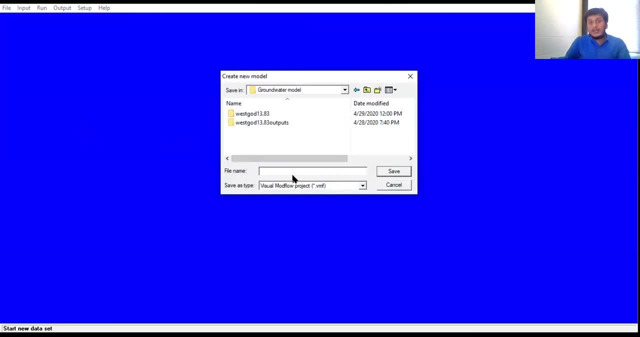 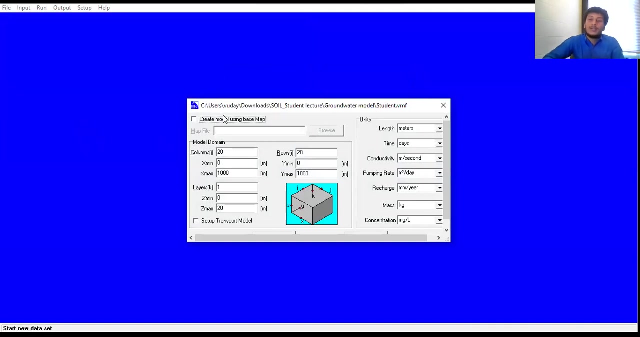 and i'll show you the outputs and all. so we need to click file, then go to new, then we need to create a folder or file, like i'd like to say here. the file name is that. so suppose, for suppose, like let's take, so, uh, we are gonna, we are gonna uh, study the groundwater flow in the far goodwill. 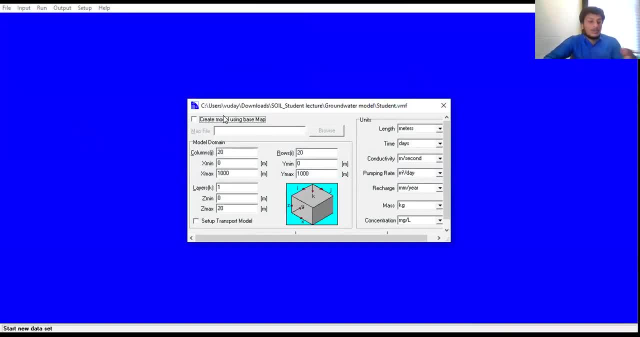 under the far girl. so let's, let's assume, uh, so to model the, to recreate the conditions. so first we need to know the latitude and longitude or or or length of the super. suppose its length is, like some, somewhere around thousand meters. so if we have base map, 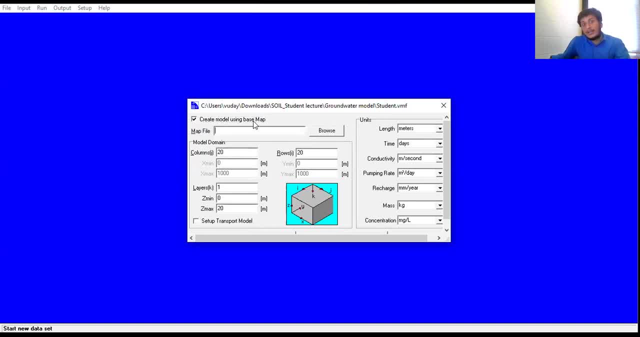 we are gonna- uh, we can, we can directly click, check it and we can browse the base map to get into, get back into the work on the on the map. this map is like: uh, so suppose in our example we said like fargid, so we can, we can get the base map by. so go to the, go to google maps. 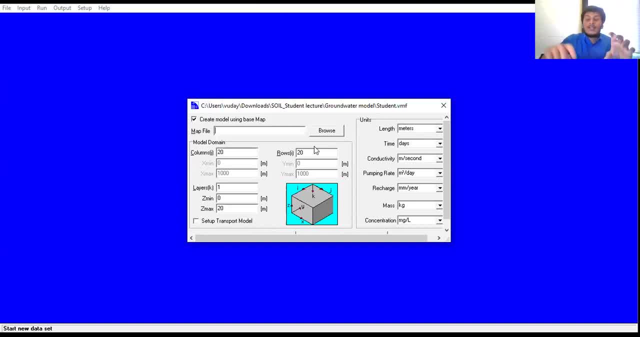 we can zoom out, like completely zoom in, such that, uh, fogged on, should, should, should, should, set on the frame. so four quarters of the phago dome should be there- and using snipping tool or any other sniping tool or other tools like, just crop the phago dome and just convert into bmp. 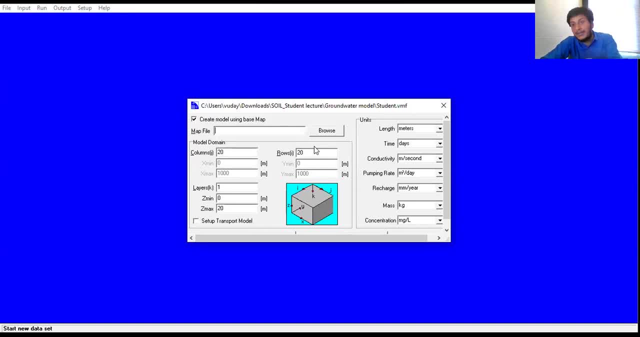 those formats are in jpg or png or jpeg formats. it won't take visual more flow won't take those formats. so if we need to convert into bmp format, which is like business format format, i'm sorry. so we can convert. that we can do using google or online conversion. be okay for it. 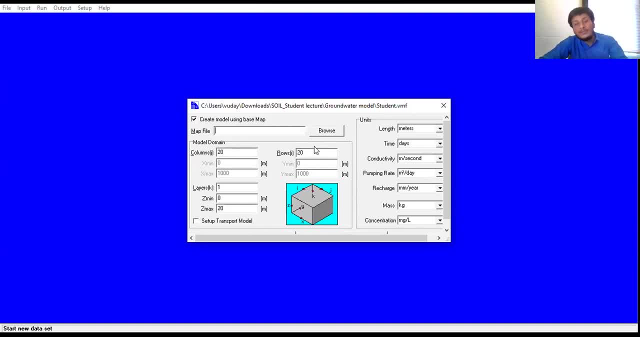 so, after converting the base map, we need to, uh, we need to, we also like uh if you want to work on the latitude and longitude longitude, or you need to know down the four corners, four corners of the uh boundaries of the uh base map, or else we can. we can measure the length for length of the length, width of the. 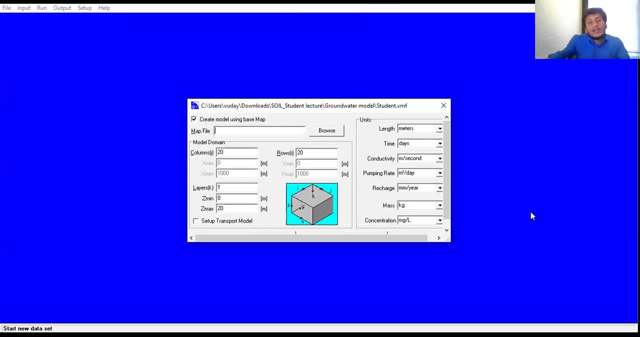 part of our rotation. so yeah, so if we don't have base map now, so i just i'll directly click the uh give the dimensions later. so, number of uh. this is the uh columns. so after including the base map, we are gonna have like we're gonna divide. 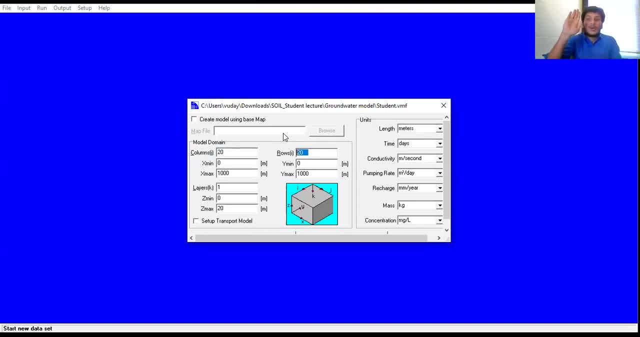 the whole area into small, small grids. so suppose this is a small area, i'm gonna a small grid, so it has set an impact for large areas. we need to take more, more uh number of grids, so we're gonna decide so. so for this example, we will say some 50 by 50 grids. 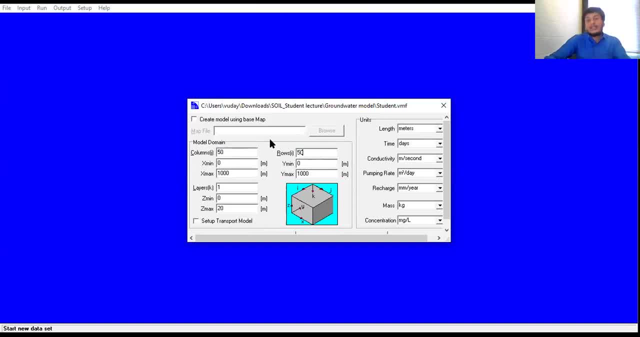 so, uh, 50 by 50 grids. it means whatever. whatever the dimensions of the grids will be map, irrespective of dimensions, we are going to get only 50 grids on the study area. whatever it is how much it is like, we'll get 50. So then, this is the minimum and maximum It. 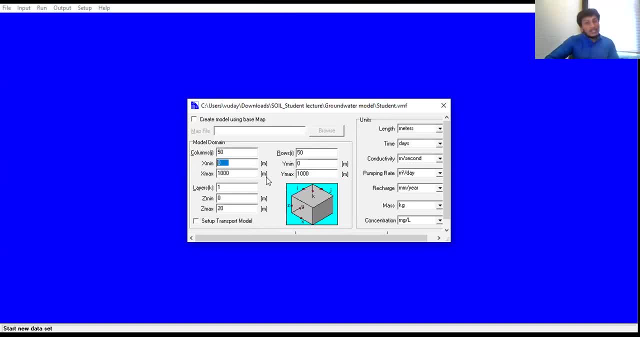 is the elevation. So to model the groundwater first, we are going to give the surface elevation. When we will be having our soil will be in different layers, So we are going to layer them. We are going to give layers in input, So to say that suppose we have a layer of 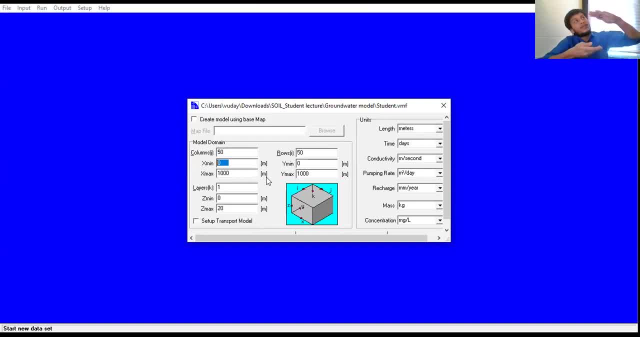 soil till 20 centimeters deep, 20 meters deep In this case our mean sea level. we have to give the elevation of the far godown elevation at the location and bottom is 20.. So we need to give X max and X minimum there. 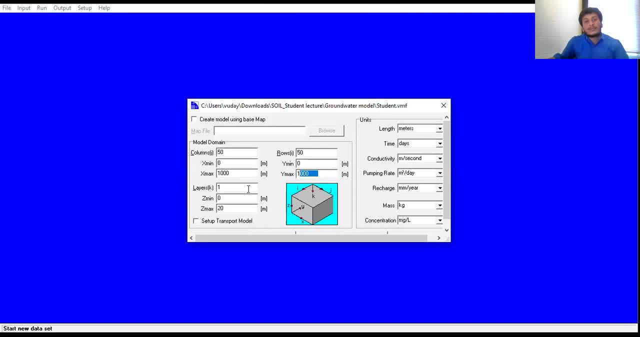 Similarly. yeah, Then how many layers we are having? So suppose in some study areas we are going to have like more than two, three layers like top layer, though suppose in some areas like sandy layer is a little like some three, four, three, four meters deep. 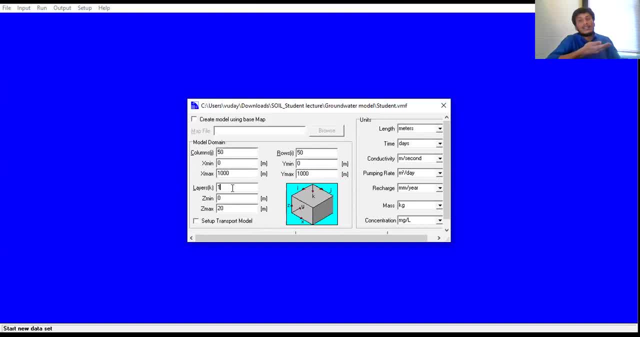 followed by clay soil, clay soil divided, followed by some granite niches or some hard rocks and all So we're going to have four, five, six, seven, eight layers. So in this case it's like we are going to tell the model that in our study we are going to create some six. 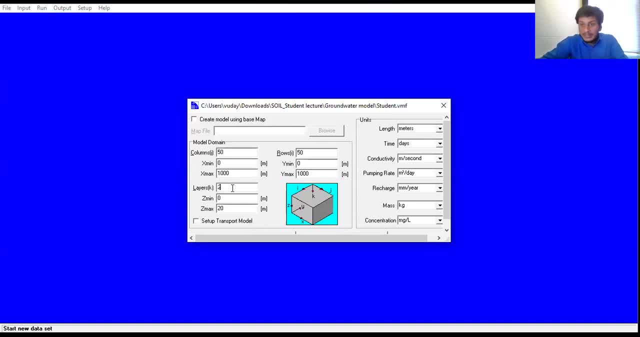 seven, eight models, For example. in this case, like you say, we have two layers, then Z minimum, Z max. It is like, yeah, it is a layer with layer thickness of thickness of the layer And X, X minimum, X max is the. is a, is a is the dimension? I mean, I mean- my apologies, Yeah- 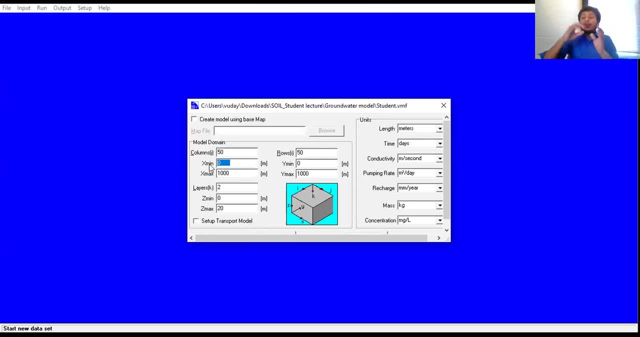 So X minimum is the if. suppose this is the fargo, suppose, yeah, this is the fargodown. So this is the length, this is the width right. So X and Y axis we are we going to give. 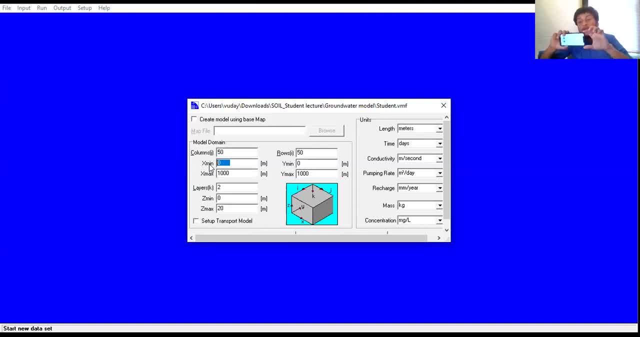 this is 10 centimeters. It is 10 meters, sorry, thousand meters. And this is two, three, 40 centimeters. It is we're going to give. we're going to give. it starts zero, zero, 10, 15,, 20, 30, like a thousand Zero, again zero, 10, 20,, 30,000.. 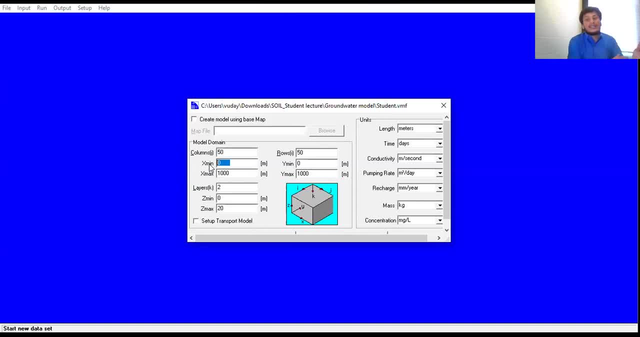 So it depends on the its we are going to give. we're going to give some readings Like the length of the field, width of the field, based on. So then, if we are going to use the latitude and longitude we are going to give, 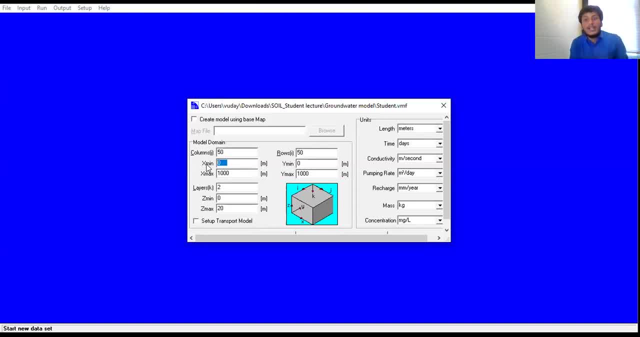 the latitude and longitude, the minimum latitude, minimum value and the maximum value. So this is 10 centimeters To Capes. we give each of this 10 centimeters, 6 meters difference value and the maximum value. That's how we're going to do it. So suppose it is, let's say: 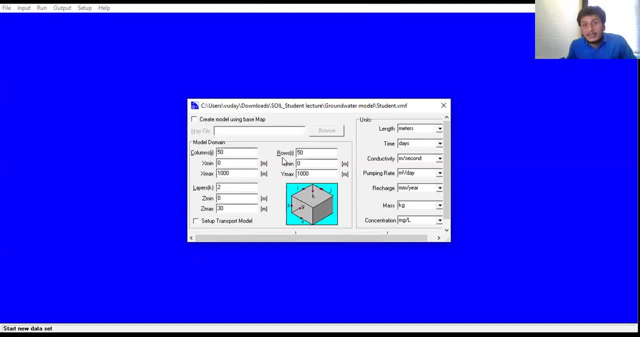 some 30 meters deep and yeah, then that's all. So our model is almost ready. If it is a transport model to study the leakage and all leakage of the flow and all like any leakage in any spillways, in those cases we can use the transport model. Now we are just 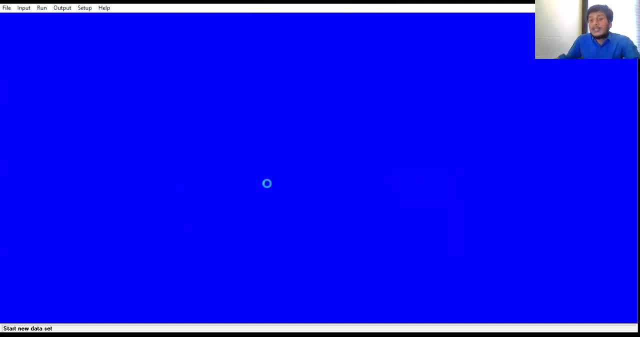 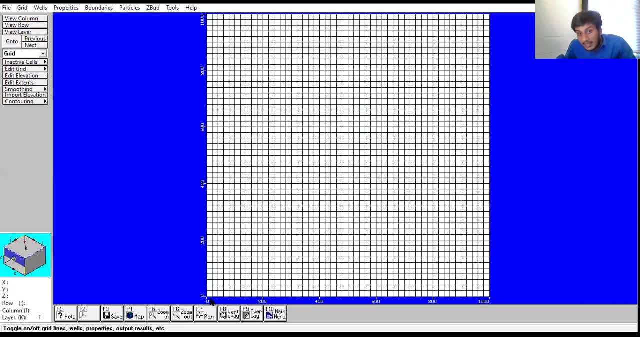 going to discuss about groundwater flow modeling. Just click create. That's all. We got the. we got our model with all grids. So you can see X minimum is zero and it went to thousand. Y minimum is zero and we entered it as thousand because we assumed that our study area is 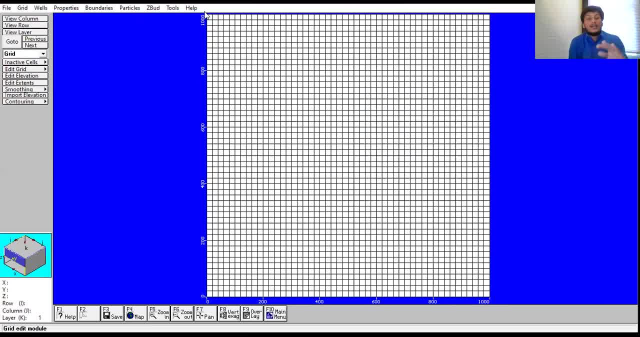 like thousand meters deep, thousand meters. I forgot to show you that, like after creating the model, we got an option to choose the units. We can use that too. So then, so this is our, our, our, our top view. I mean, if this is, 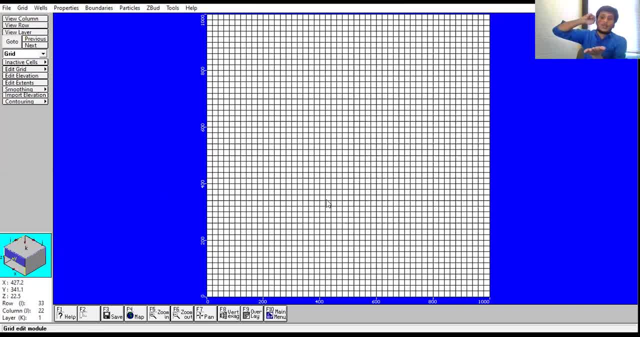 the Fargo dome. this is the base and this is the top of the Fargo dome. So when we see from the top satellite view, Google maps, you can see the top face, the face of the head of the Fargo dome. This is one, this is the one. So we're going to so slowly. 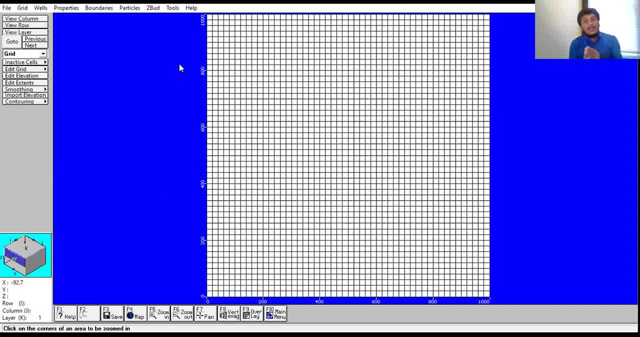 step-by-step. we're going to do X, Y, like first we are going to do the layer thickness and all. Then we are going to locate observation wells or piezometers, whatever locations, at different locations and followed by other properties. So now we created the model. We created the model. We need to view the thickness, the 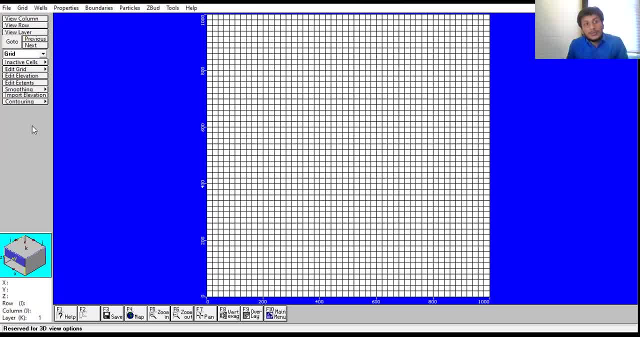 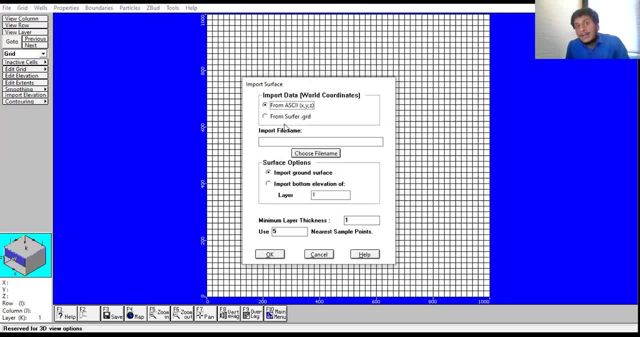 millimetre Layer elevation. To do that, we need to import the elevation. Import the elevation could be like we can save in X, Y, Z or Surfer is a software right. I hope you guys are aware of it. 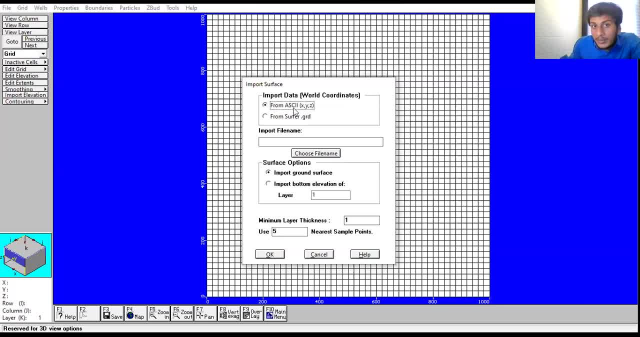 So in this case, we are going to give the, the first one, I mean from AC, X, Y, Z- right. So, for example, you can go to the soluble object. It is this, it is, this is the this. 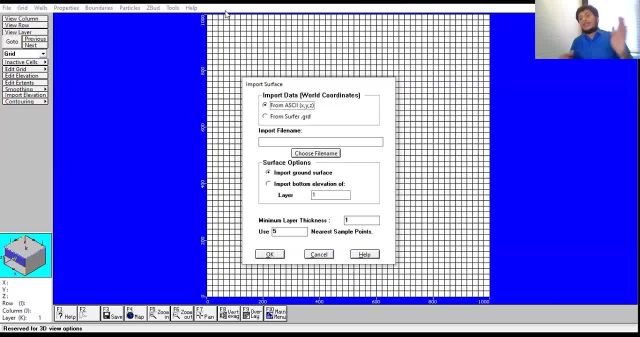 variable, right, It is this one. So we are going to do Y Y Z, X, Y and the second one, and this is the surface elevation. All right, We will give X Y Z, X Y Z. So we are going to do Y Y Z, Y Z up to: 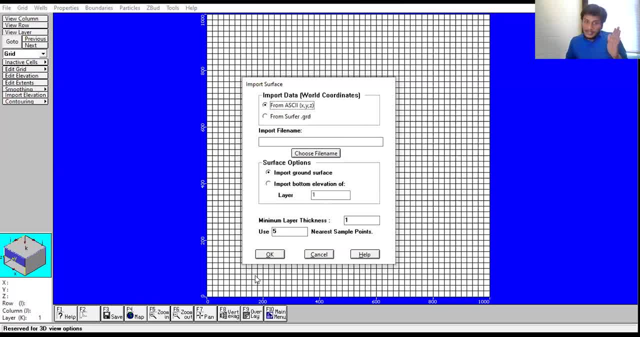 this value. Now, this is not the center of the object, It is this point on the top of the surface. It is an object. We are creating this vector. In this case, we are going to, we are going to write this vector here. This vector is: 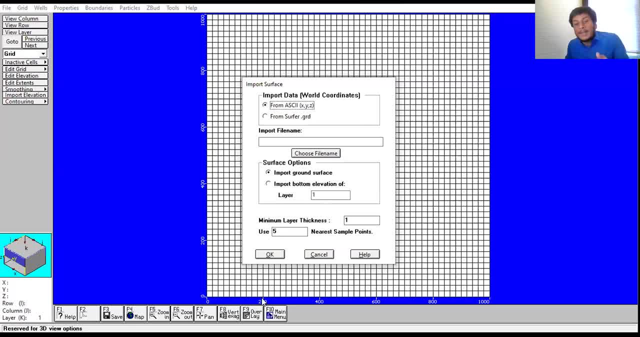 suppose to give the elevation. here we need to say 200 comma, zero comma elevation. suppose the elevation at 200 location is 20, then we will say 0, 120, which means 0, is the sorry 200, 0, 20. this x coordinate is 200, which means length. then y coordinate is 0 and 20 meters at this location. 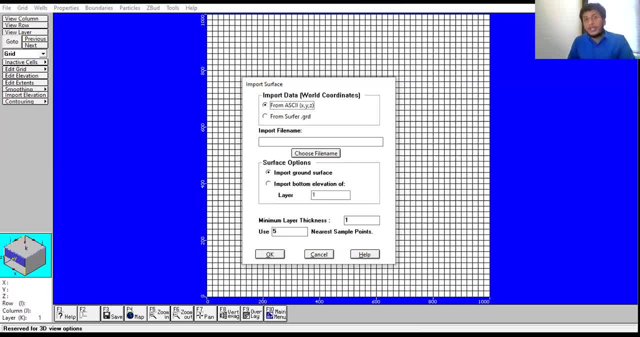 the surface elevation is 20 meters. similarly, we need to give it randomly as much as possible. if we have more numbers, the more accurate data will be having. the reason behind this is so, after doing that, we will say this is the ground surface when we are going to do the 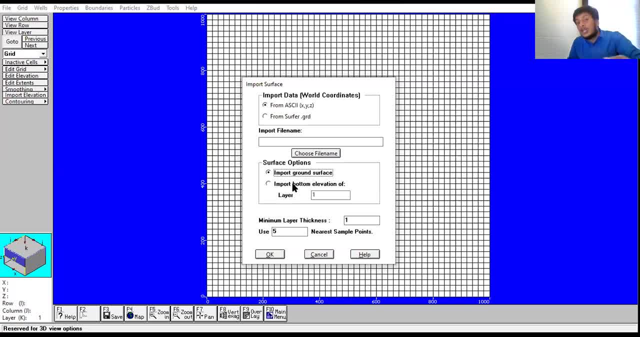 ground surface. we have to click it. after giving the ground surface, we are going to give the elevation or thickness of the next three surfaces, like soil surface, sandy soil, clay soil or other soils. so to give the thickness we need to say import, click the import bottom elevation, then click which layer elevation are we going to incorporate. then we 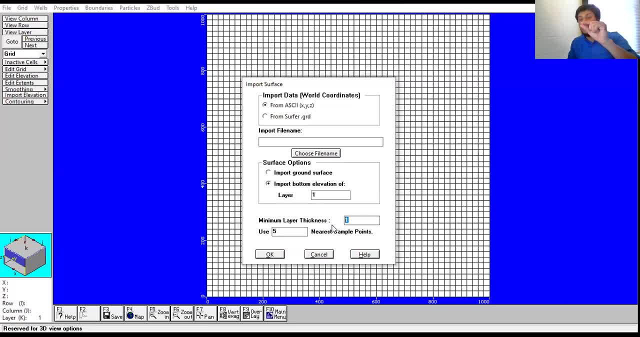 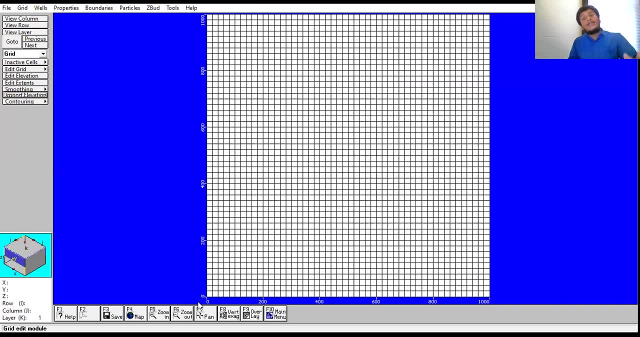 would say the layer thickness. it's kind of like how much thickness you want to see the layer. that's all then then. so, after giving that, suppose if we have two, only two, three values, it will definitely take it, but we will not. we will, we will fail to recreate the real conditions, because if we use some two locations, 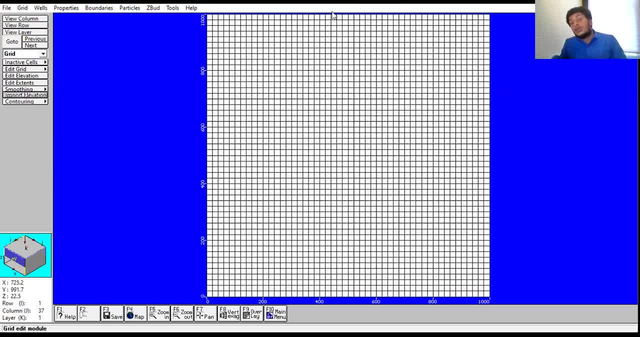 it is going to take, do the interpolation and it will give same value from each grid. so suppose if we give 20 and 40 here, it will do interpolation and it will do. if we give thousand values, it would take so that that that would take. so that that's how it works. as many points will. it's better to recreate the location. 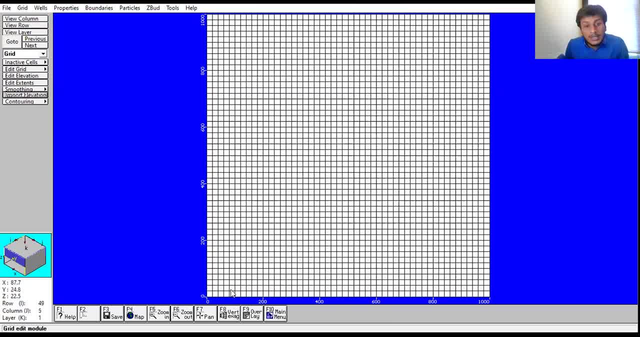 now we need to check whether our data is correct or not. so to do that, just click. like you don't need to click, just go to the uh, any known coordinates, and just place the cursor there. we can see x, y, z here. x is the x location, sixteen point, six y location and z is twenty two point. 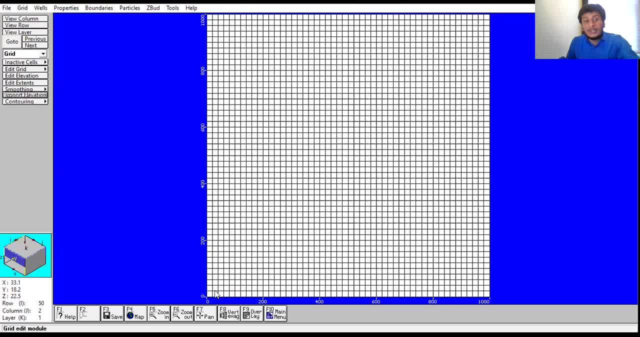 five, which is like didn't do anything. so that is how it's showing 22.5 everywhere. so that is how it works. 22.5 so slowly. we need to import the other layer, other layers, then we are gonna. so, after importing things we can, we can view them. i i'll show in the in the existing file later how to view. 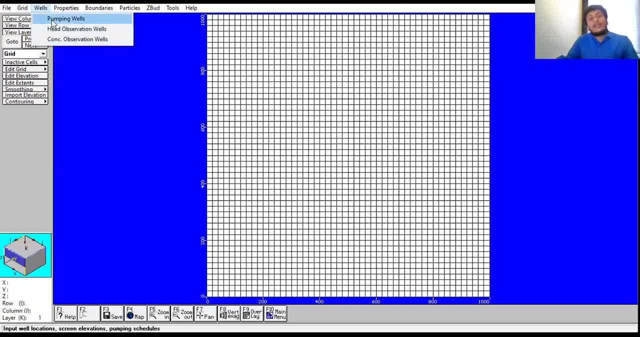 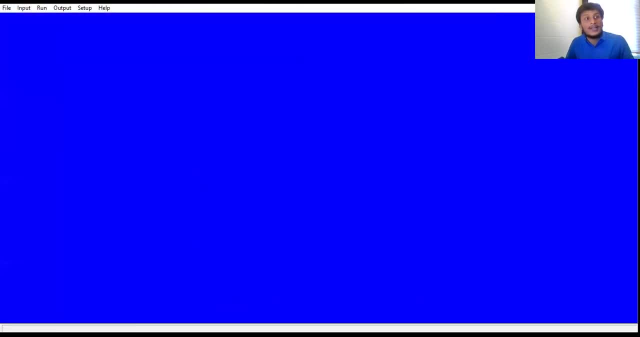 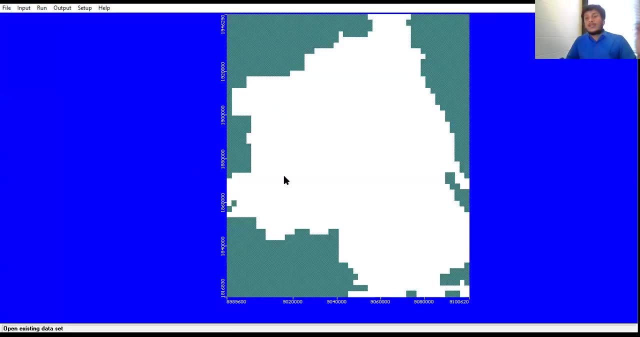 at all. so then we're gonna click some pumping wells, just save it properties like we have. i think it's better to in the existing file. so that i can show you better, i'm going to open the existing file. this is one of the existing file, like which. this is a base map. actually i, i just uh. 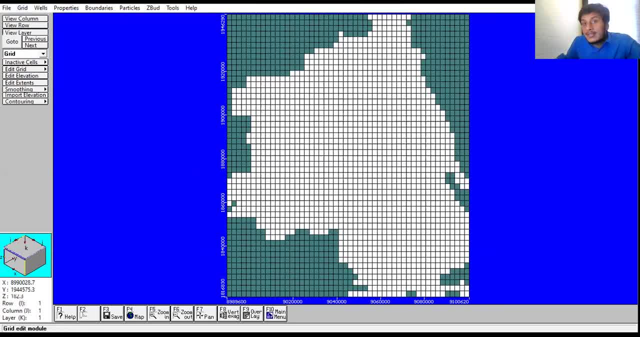 i'm going to go here so yeah, so this is, uh, this is the base map. so i would like to delineate my study area. so i used inactivate cells. so we have mark single, so if we see market, those cells will get inactivated. so so that is how i delineated. suppose, if, if this is the file dome, i'm gonna 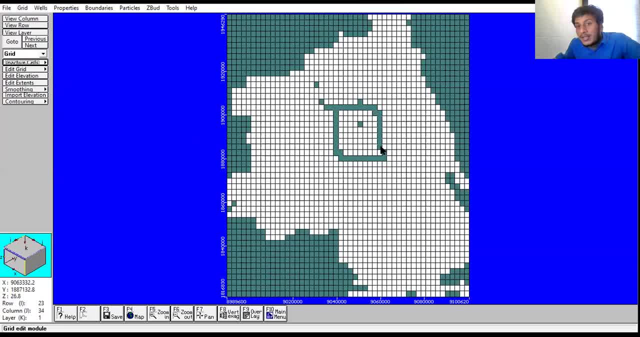 delineate this. so this is my study area. i'm gonna walk here. this is like excess power, excess portion, so i'm going to see what i'm going to use them. so that is how we delineate them then. then you can see how the xvc is changing. you can see the elevations here, how z or it is. 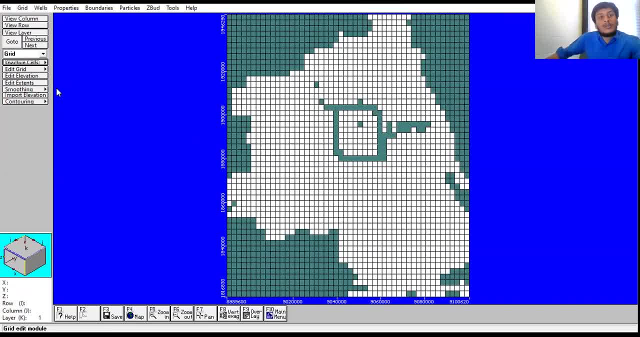 changing 3.8, 9.4, which has high elevation. so then we are going to, after importing the elevation and after delineating, we will import the elevation. after importing the elevation, we are gonna pumping wells, pumping well data. we need to save it because I don't want to save it. 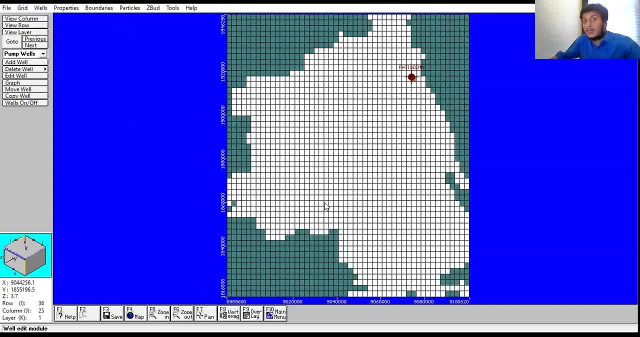 because after running the model it may cause error. because we have many observation wells here, To let you know. I just did that. I didn't say that Yeah, to add the pumping wells. we'd say this is a. in my study there is a pumping well which lift the water from. 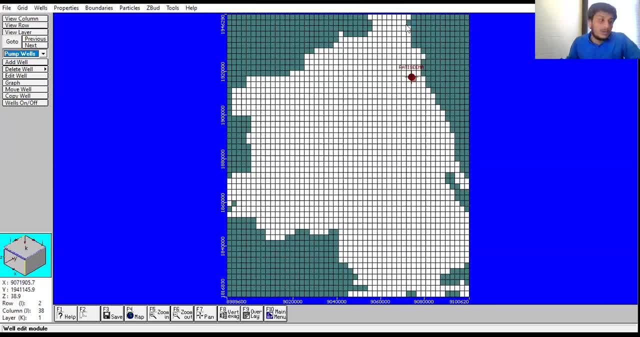 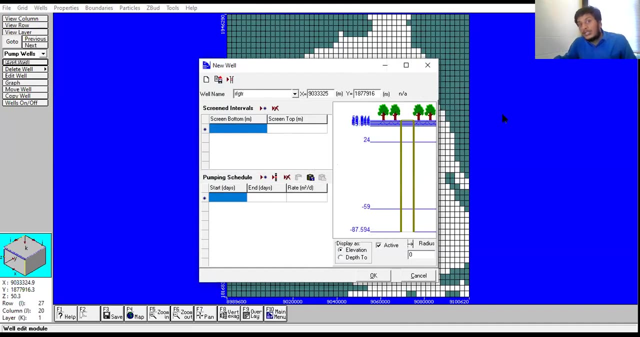 one river and will? I don't, it will discharge everything in another river. So I just addressed a pumping, just click. add well, whatever it is, based on the location, We know the location. so, based on the location, just give the well name, then coordinates, because we choose. 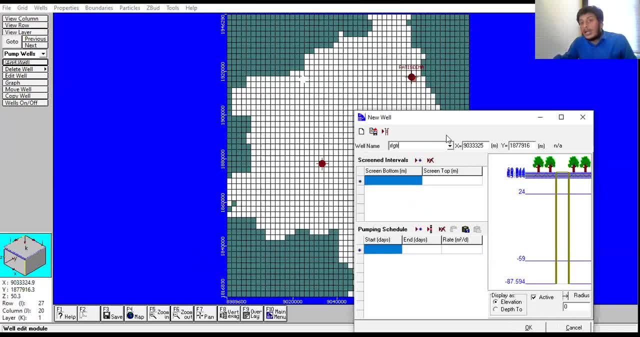 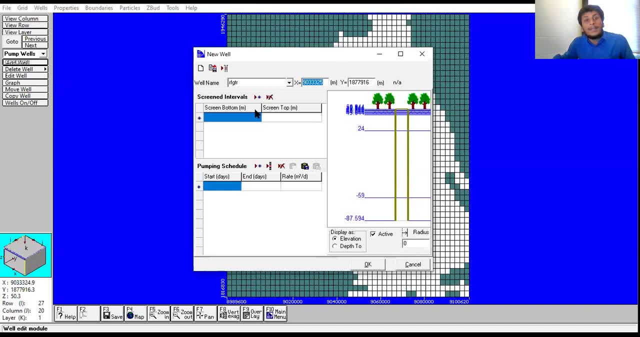 we can see the coordinates here, this x, y, z, So I will get the coordinates. If you want move the well, then give the existing coordinates. correct coordinates of the well, then, screen bottom. So, while giving the observation wells and pumping well data, we're going to. 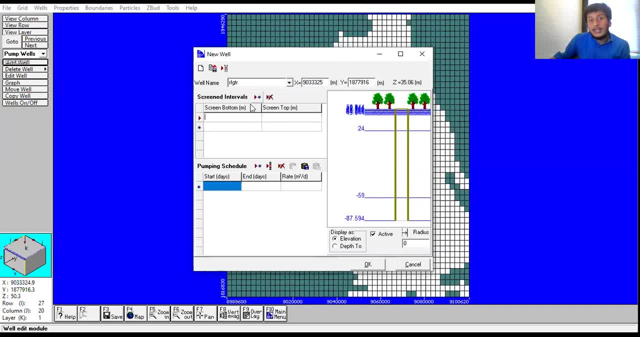 give to, it will ask: the well screen. So usually suppose the mean sea level is it's zero, right? So if you want to give the top- from the top I mean the depth- what you want to give is the water, groundwater depth. we need to choose it. We need to give the 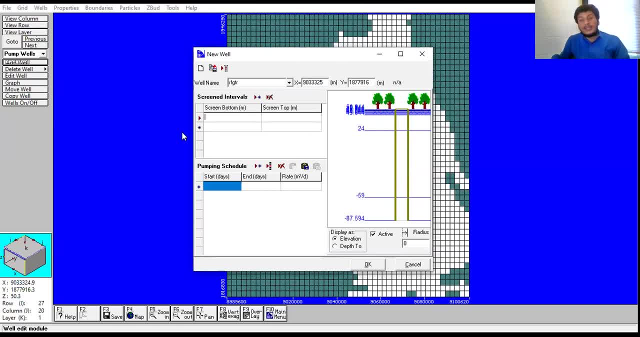 groundwater depth from the surface surface of the surface. That is how it will take, So we need to give them in the surface or this is the elevation It takes. from the elevation. It is depth, which means we are going to give with respect to the mean sea level, If you. 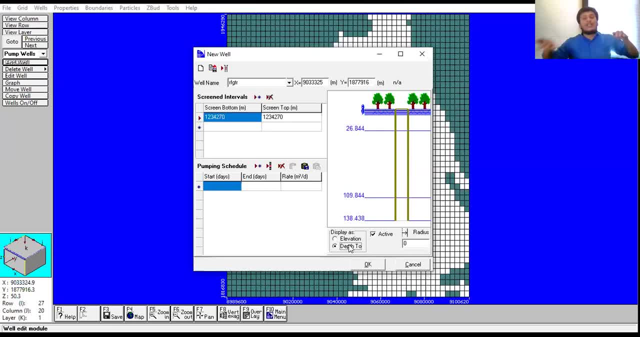 want to give the water depth with respect to mean sea level or surface. based on that we can check it, This elevation and depth. Then we can check the elevation and depth We're going to give starting day. Suppose in day one it is zero to day one, And how? 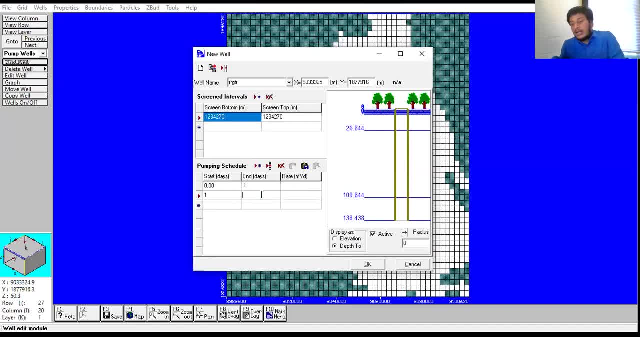 much, how much rate it took then one to 10 days, how much it took. So suppose like this: so in 10th, from 10th day to 650 days. So that is how we are going to give, we're going. 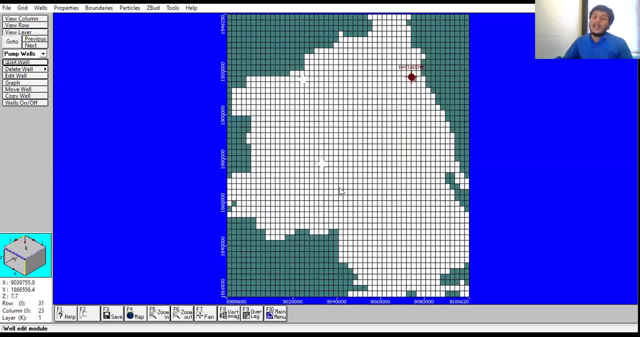 to give the pumping pumping layers. So usually we'll be having some pumping wells or survey pumping wells or other drainage, and all Drainage- I mean drainage canals. we are going to give them as boundary conditions. So if there is any pumping well in our study location, we're going to get it. So next, 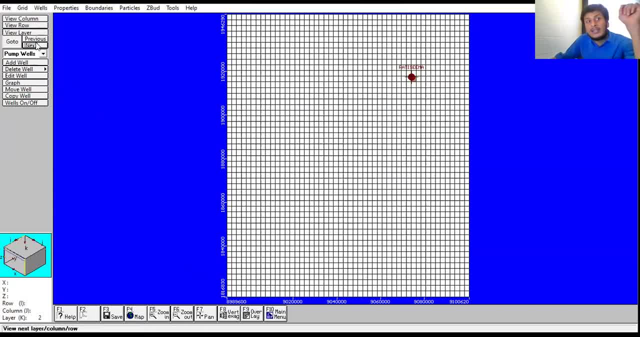 click next It is. it is in the second layer, It is in the third layer, Like so my study, my study area is, has around, I guess, 10 layers, So I am having 10 layers. So if you, 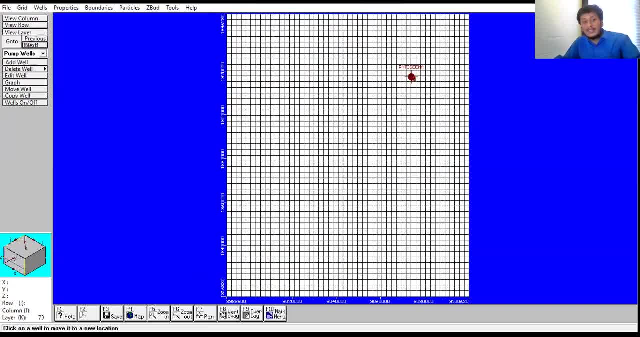 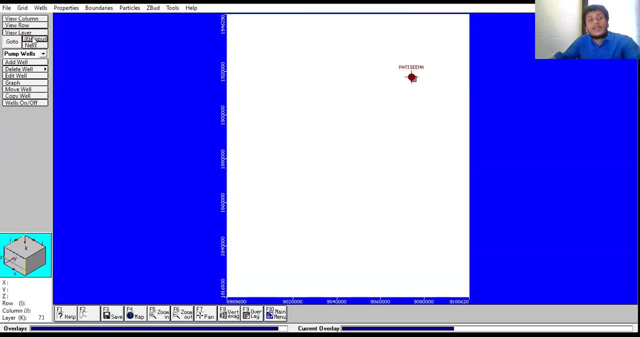 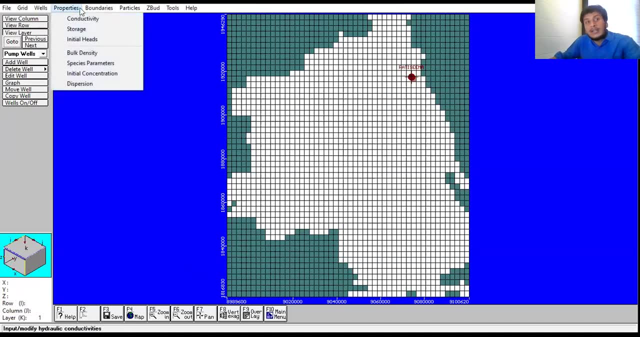 click next it will go to the. it will take to the next layer. third layer, fourth layer: This is the seventh layer. This is the eighth layer You can see here. this is the number of layers. That is how it will do. Then, properties like wells, head observation, wells- we are. 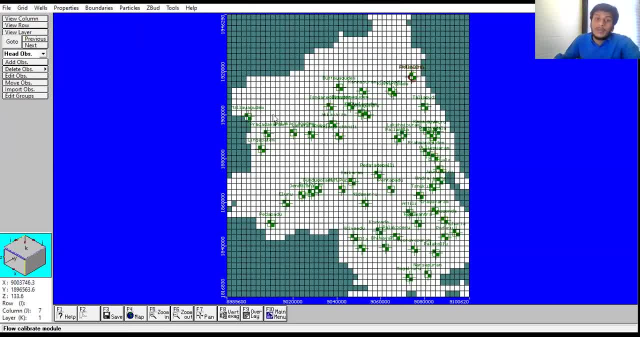 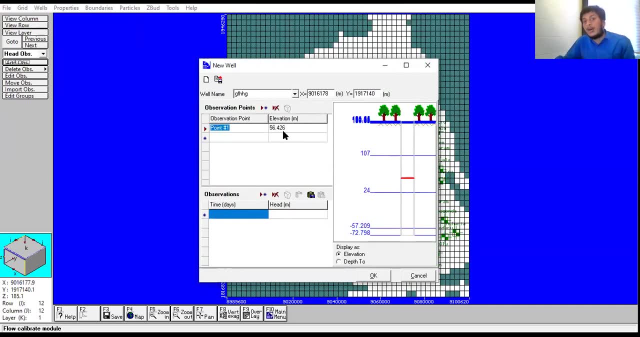 going to add observation wells. So in my study area we are having somewhere around 51 observation wells, So just like add observation. well, the same way We're going to name. name it u, x, y, coordinates, observation point. It will take automatically, So time how? 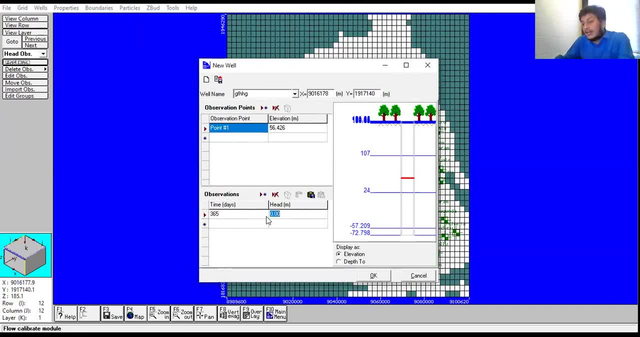 many days. So first 365 days. This is the head observation well. head is 9 meters, 6 meters deep, Then from 600,. next we are going to add observation wells. So we are going to add observation. 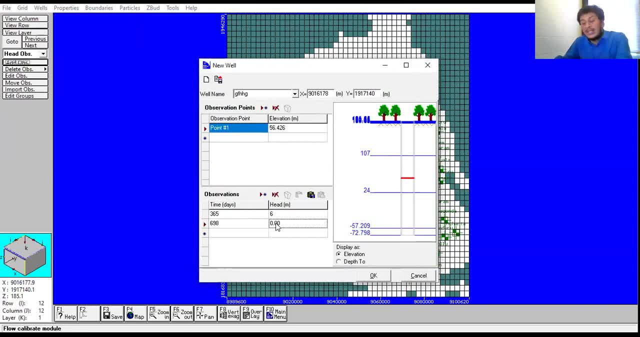 wells. So in my study area we are having somewhere around 51 observation wells, So just some 698, 365 to 698 days it went up, Other days it went down. So that is how we are. 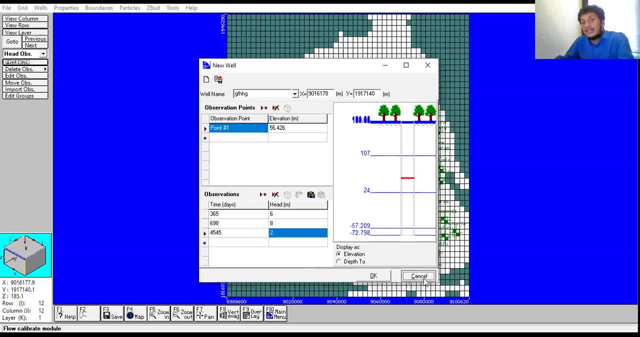 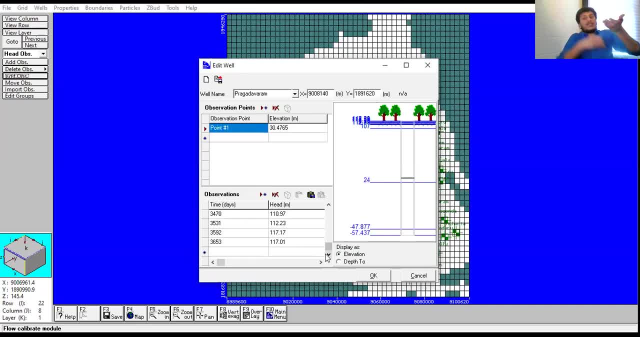 deeper. it's going down. it is 108 meters from the top and then it went 109 meters, 110 meters, 140 meters, 170 meters. It's going down. That's what it's showing. It's saying that it is from the elevation. That is why it is from the elevation. 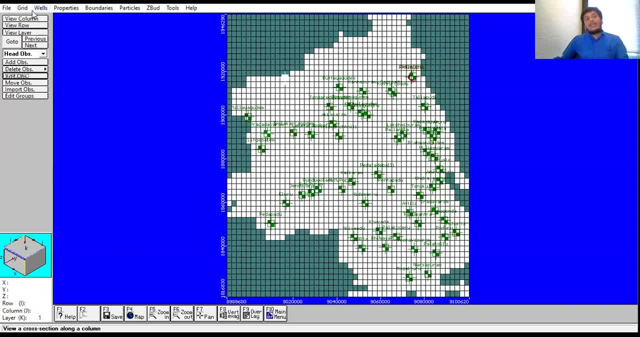 So after assigning the observation wells, we need to say concentration observation wells. this is for transport models. If you want to address some spills and all, we are going to use that model. So then this is the main part of the study. we need to address some. 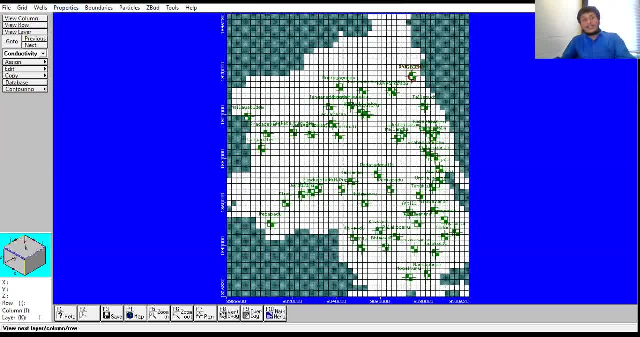 properties like hydrological properties. so conductivity. So we can assign the hydraulic conductivity in layer wise, polygon or whole window or single. Single means we need to click somewhere and it will say how much we need to give the hydraulic conductivity. 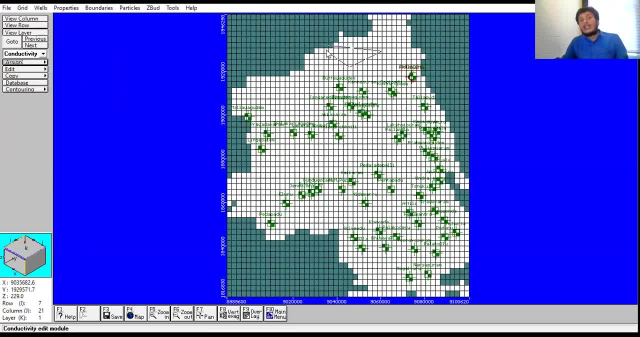 For to assign the polygon, we need to click select some layer and we would say in this location, Because in some very big area, suppose for suppose, if we are going to do for fargo, whole fargo soil, if suppose half side is like some other soil, half side is fargo clay. 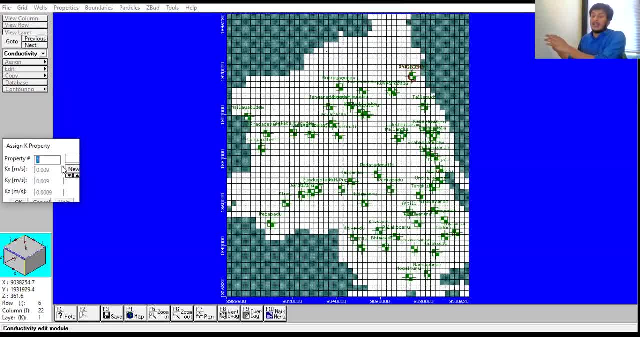 soil. In this case we are going to give fargo clay soil one hydraulic conductivity, the second layer as a second hydraulic conductivity. That is how it works. That is why we need to use the polygon. Then storage: How much water storage and all? I am sorry, not storage, storage capacity and all this. 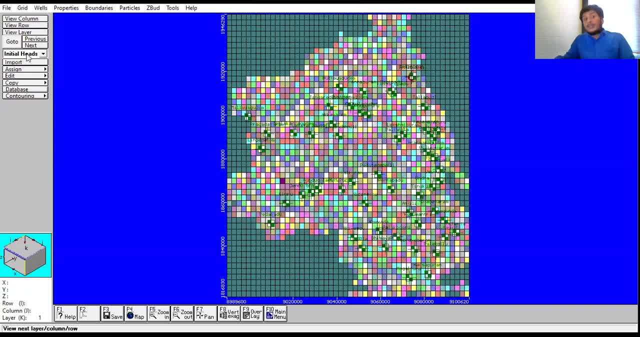 we are not going to give that initial heads, So after giving the. so this is completely based on all well observation data. So we gave the head observations right. So based on head observations, this made this graph. it gave the head observations for each location. 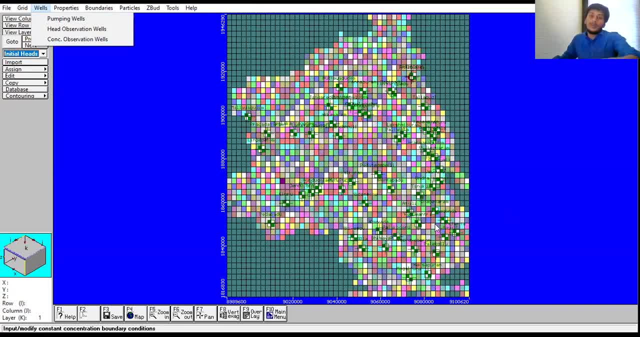 each color represents. So that is how it works. So it made the initial groundwater flow condition for the model, Followed by initial heads of this. this belongs to transport models. So now we are thus: we created the soil surface, we created the surface or location of the 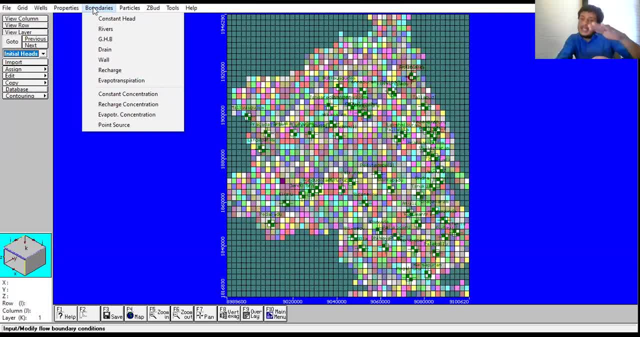 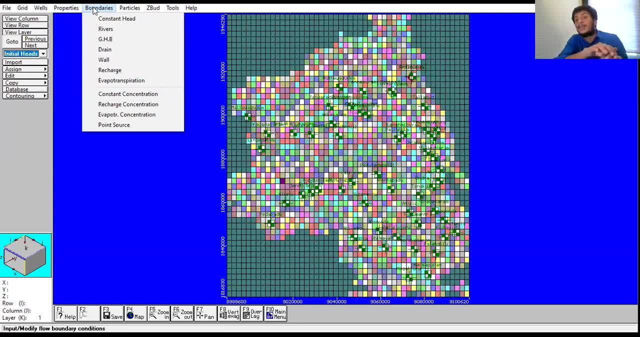 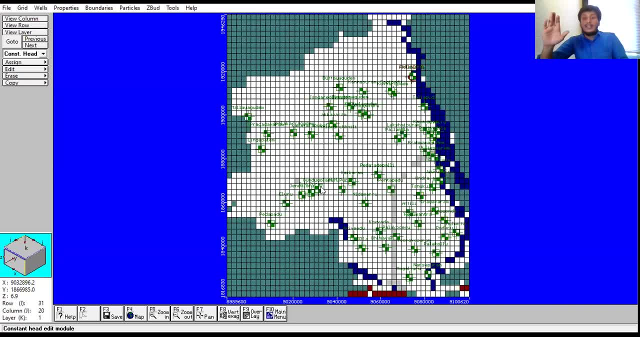 well data. Then we are going to address the boundary conditions, which is very important now. So boundary conditions: they will help us to understand, to study the. so boundary conditions means any river drainage canal or rivers, drainage canals, rivers, seas or any water. 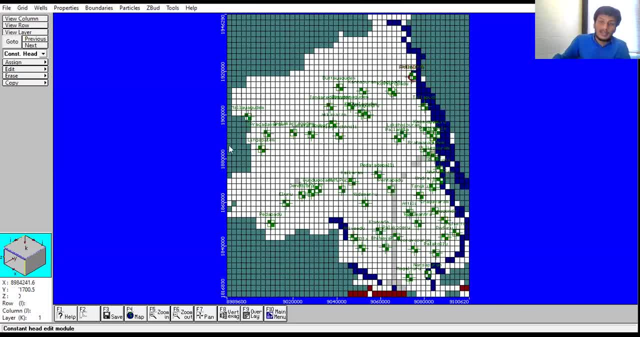 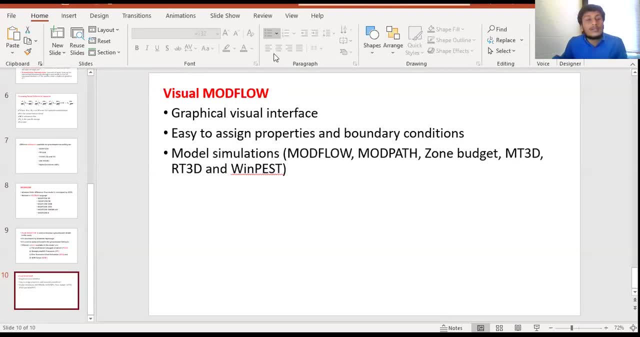 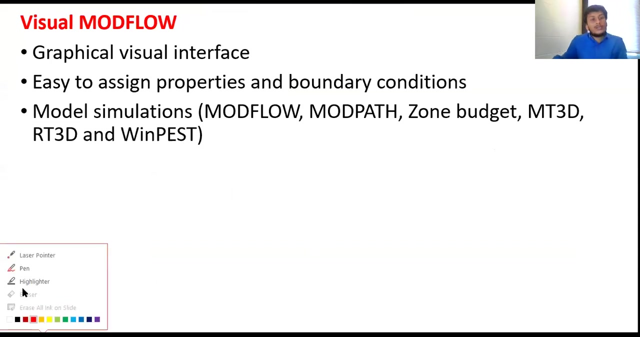 surface bodies all comes under boundary conditions. So in my study, in this study. so this my study area is located in- I think I can explain it here- So in my study area. so it is my study area. 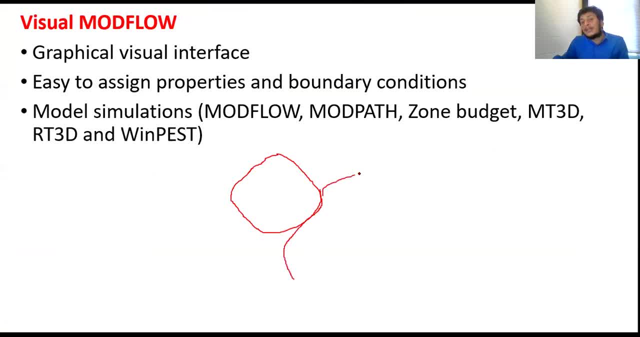 So this is Bay of Bengal Sea. We have sea here, We have a river, river Godavari River, River Ye here, And we have another river here, River Tu. So that is, this is my study area, And it has a biggest, longest lake. like good water, like pure water lake, Then this is: 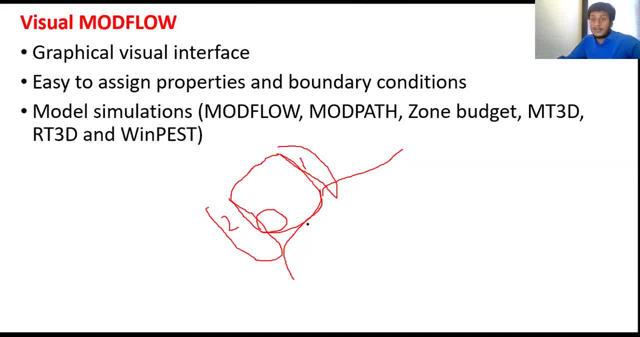 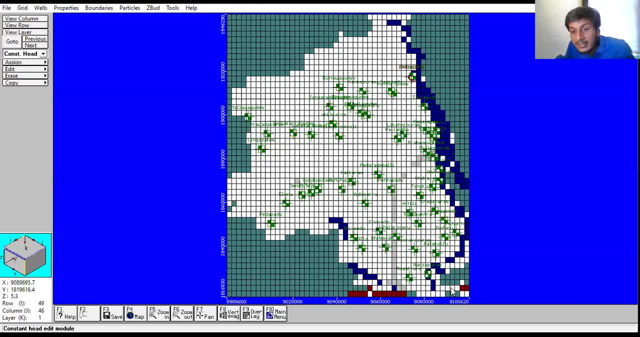 So I give the red color represents the sea in location. it's Bay of Bengal, And I gave it as if you, if you go and see there, I said its head is zero because it is sea. Because if we we read that, then then just it is actually all green is in this. 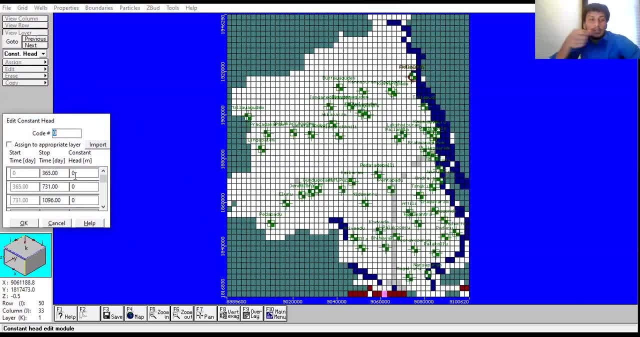 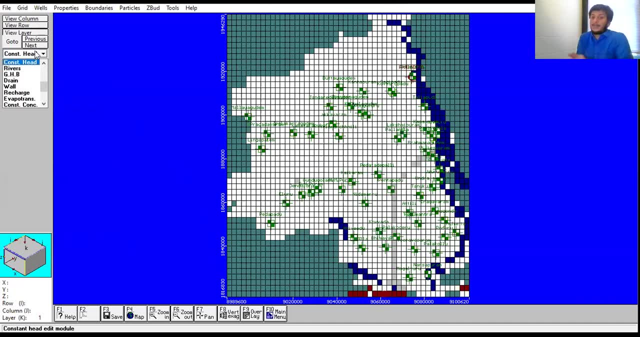 c, it has it's, it's, it's, it is zero. obviously it is. you know its head is zero. then i assign a. this is constant head, which means c, constantly, which doesn't change. we need a constant head. so that is what i made here. if it is, if we don't have constant head, we would say some, any, what? 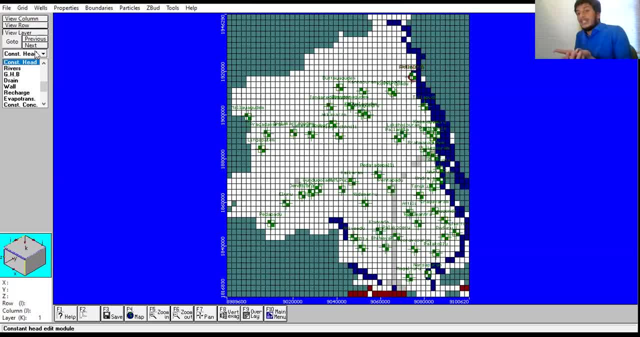 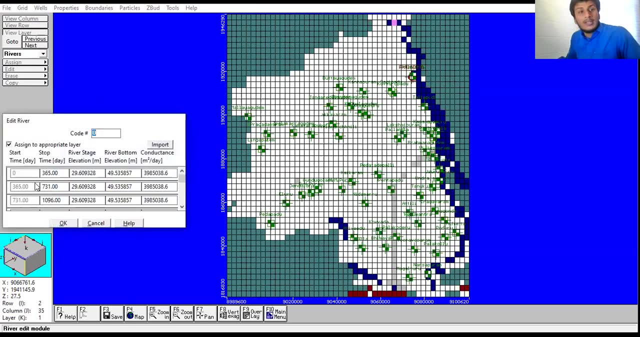 existing water body, which which which won't change forever, so we could say we could address it as constant. then, coming to the reverse, this blue layer shows the river blue river section, so i gave it so, from starting day, in first stage, zero. in the second day, 365. the reverse stage elevation. 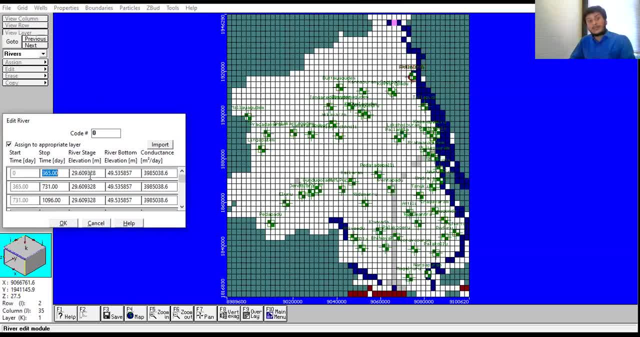 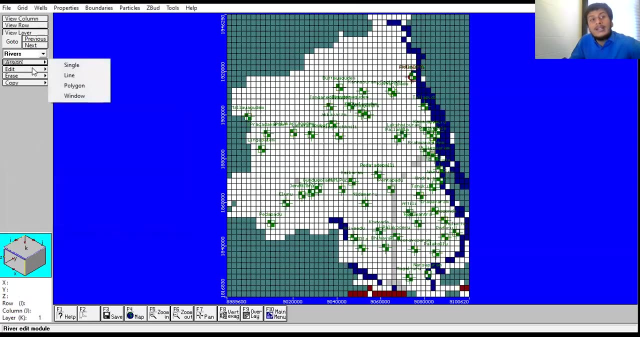 elevation at that location, and this is the reverse stage, the bottom. and so, to give the uh, to address the, to recreate the river location, we need these values. we need these values to recreate the model. so then, so i created, i allocated the, assign the river such a way that 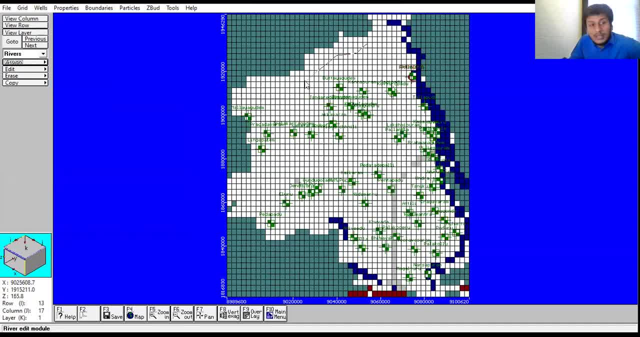 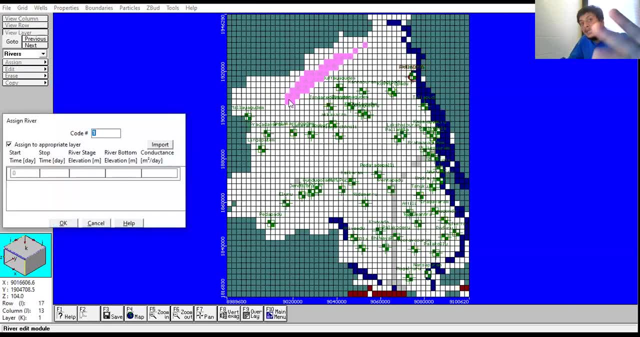 suppose, like this i arranged. i mean based on the x- y coordinates. i followed and i sent a river and i right clicked it. it means my river layer. i allocated the river layer, so i need to say how many days? 365 days, what is the river elevation at first location? and 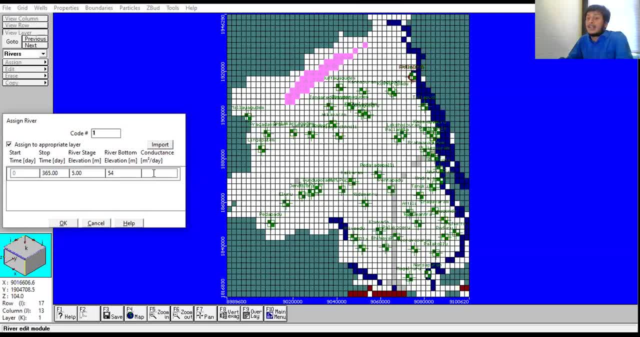 the river elevation at the bottom location and its conductance. conductance: there is a formula to calculate the conductance. so we have to calculate the conductance and i assign the conductance. if suppose then i could click enter to assign, because it's not i, i have. 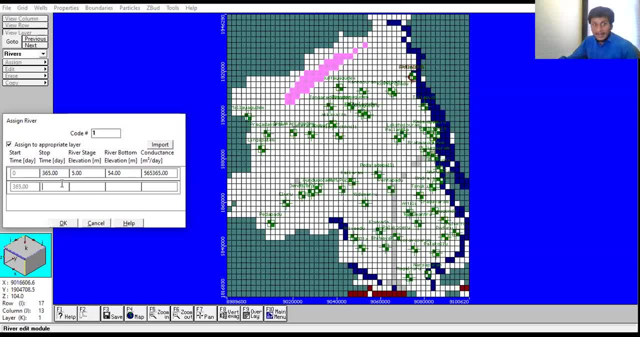 five, six years data. suppose, if i have seven, eight years data, i would say for first year how much it is second year, if i don't have year wise data, if i have together seven years data, then i'm gonna give like seven year how many days for seven years i'll assign. 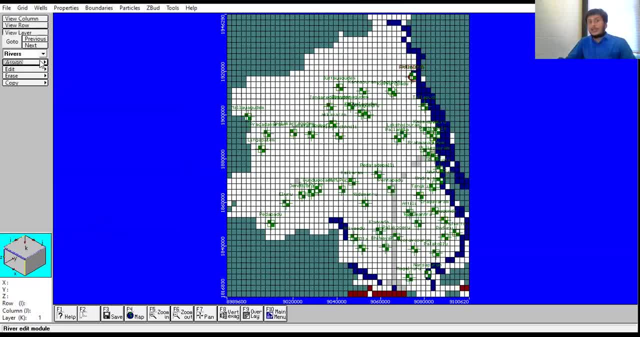 some some days there. that is how we can. we can assign them. after reverse. i assign some drain, this image, color or whatever it is. i guess color, yeah, this. so this represents the drainage. this is a drain canals. there are like a few drainage canals over there. 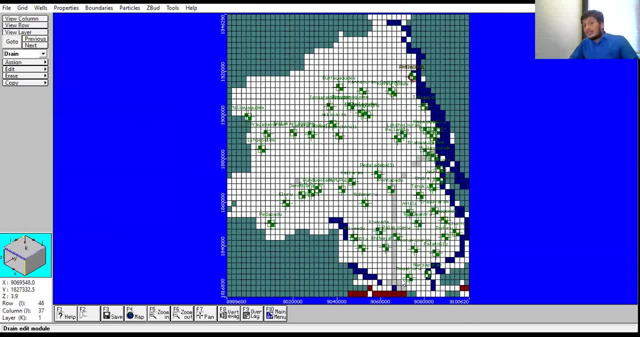 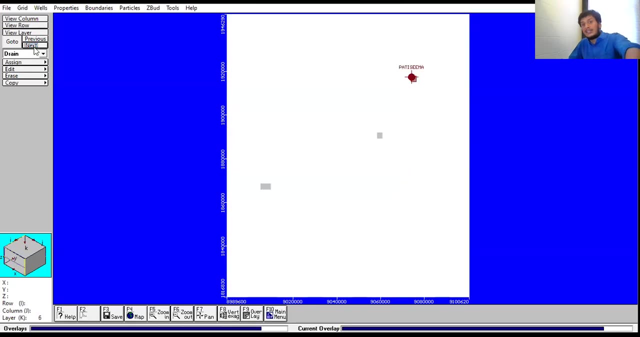 so i, i just assigned them this: directly drains to the sea. here, i just made it, i have assigned this and, uh, i have a water canal here in this direction. this is it's there, right, it's elevation in it. you can see the same assignments in the. in the next layers you can see the footprints of the river, like. 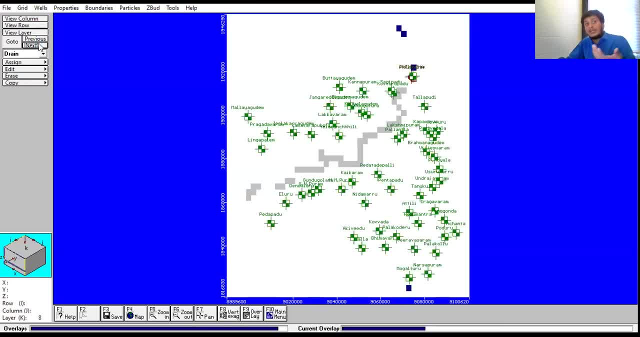 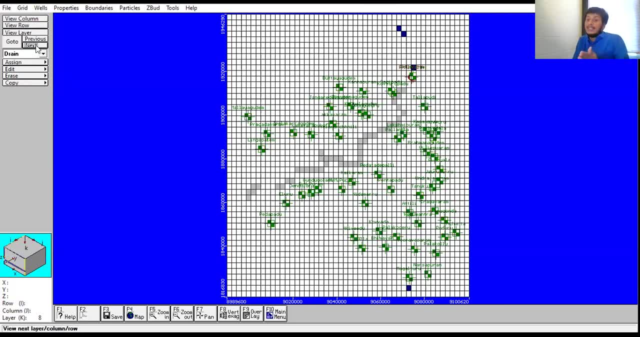 the canal you can see. so this canal, because those based on the elevation we can see. so this is the, this is the drainage canal, which means so canal has its its bottom surface, like elevation of the surface. so based on the elevation it will go and sit in the layer, suppose in the top. 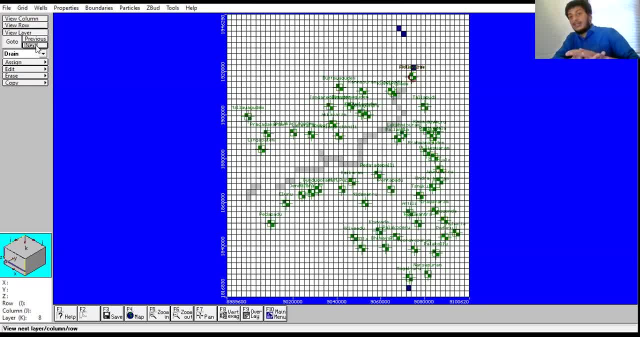 elevation. the elevation is higher than the, the, the elevation of canal. it will go and sit in the next, second or third layer, so that that is why, uh, we couldn't see the uh river. oh, i'm sorry. can all in the in the first river say: go to first layer, so this is the river? then i have saying the drying drain, drainage, then recharge. i need to assign a reason. how much region is that so from here- behind me- here is the lettuce- allows me to query water, for that is it to gross by adding water, and much better, 12 years earlier. i need to assign a region. how much here is that? I don't mind so, but can you exactly assign how much? discharge. i mean, do what you have as your spinner later on. if you finish this up will be fine. so without that you've done that already. so usually go to the other. on the bluffing story, basically, when i tell you that don't, so go to component view, then which are both of them? then I charge and you're going to a channel, the one that is instrumental. 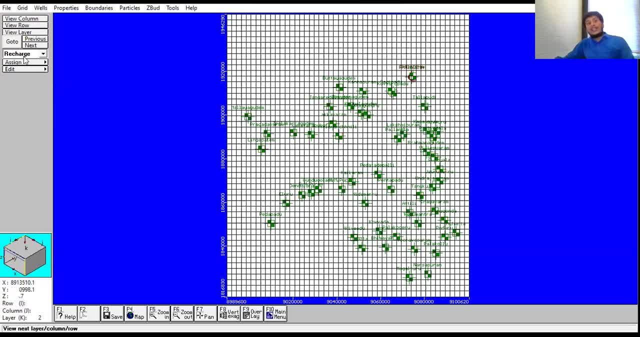 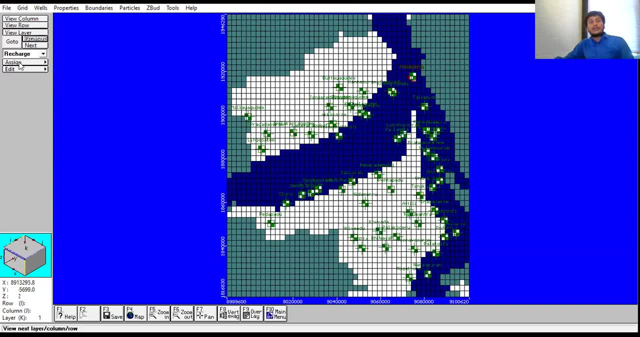 So from the, from the, from the. so to assign a recharge, single or polygon. so yeah, so I have from from. in this study area we have so many rivers, sea and and a drainage canal, So I assign the. 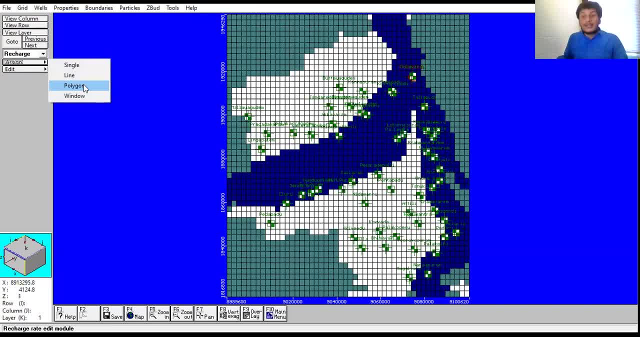 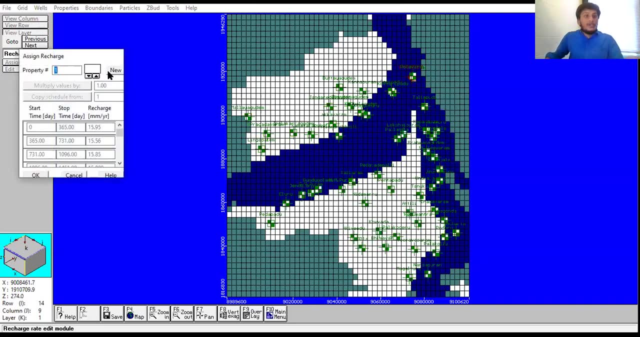 I assign the, I assign the recharge for each thing, each location. So suppose I would say this is the. I have assigned here property of a, like I would say, new color, because already single blue color represents the recharge from other river. So let's say: stop day first day. 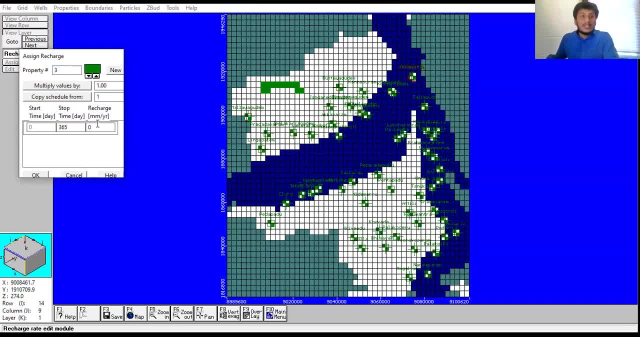 it's so total days could be 365.. Then I would say: how much recharge? calculate the recharge. again, we have a formula. so using the formula we need to calculate the recharge, Then then assign the, assign the. 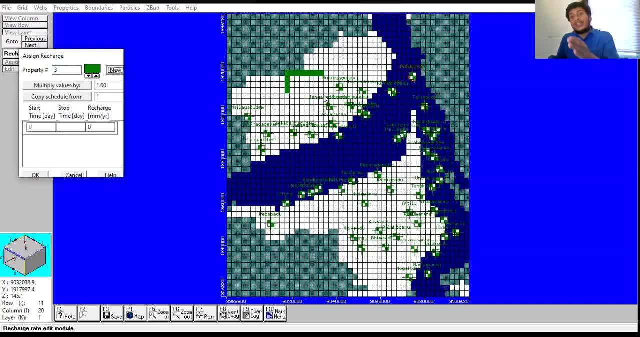 then assign the. if it is, if the recharge is same as one, you can say like no, it's, my, mine is the same, my recharge is same. or if you want new, you can say: 36 degrees, how much is your recharge? sum 56,. okay, what I say I don't want to save. 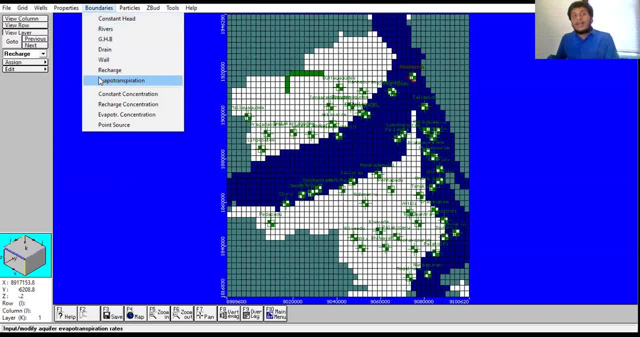 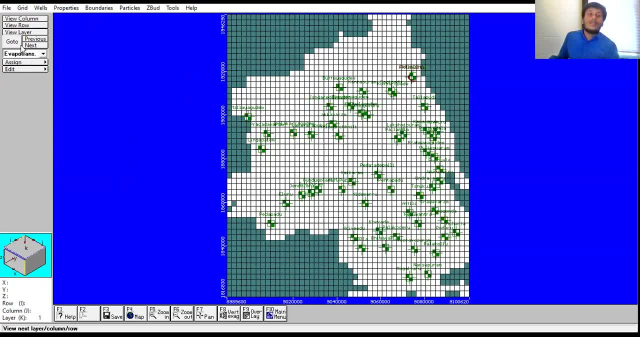 this. so I'm not going to say this. I think that's all. yeah, So we are going to give evapotranspiration in this location. So after giving the evapotranspiration it will say: okay, that's right. 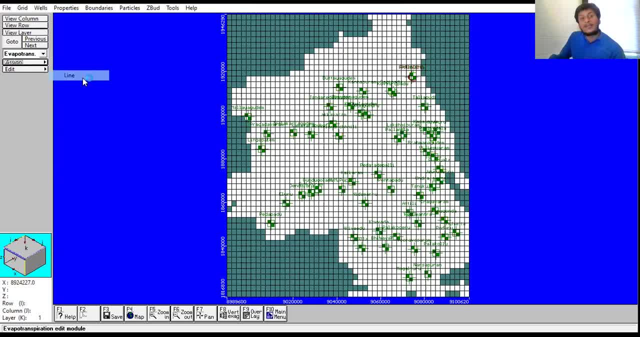 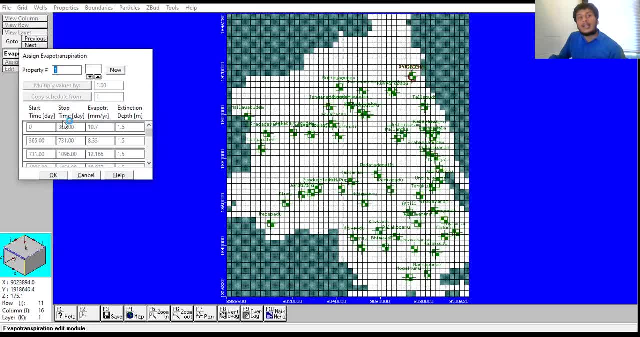 so evapotranspiration, we need to assign it. Yeah, so it doesn't like stop there, stop there. how much evapotranspiration, evapotranspiration is there? is there any? okay, so evapotranspiration, usually I took. 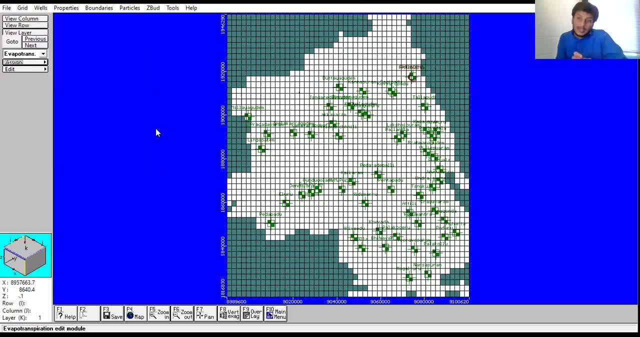 10 percent of the rainfall. so the annual rainfall I measured. I got the annual rainfall data from the government and I tried to measure the. I tried to take 10 percent up. that is how I made it. So it's not there. I didn't save it. so after this, after assigning all these properties, 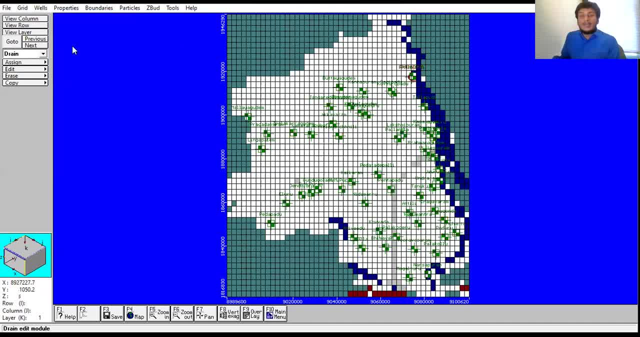 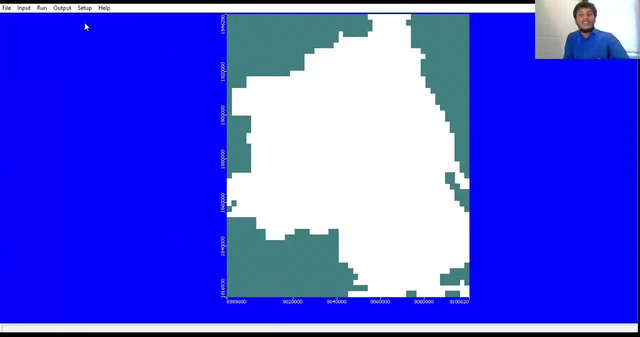 we are almost done. we are able to run the model. So now just go to main menu, and here I didn't save any edited data because I just wanted to run my model safe, without any errors. that is why, but usually when we are changing from section to section, 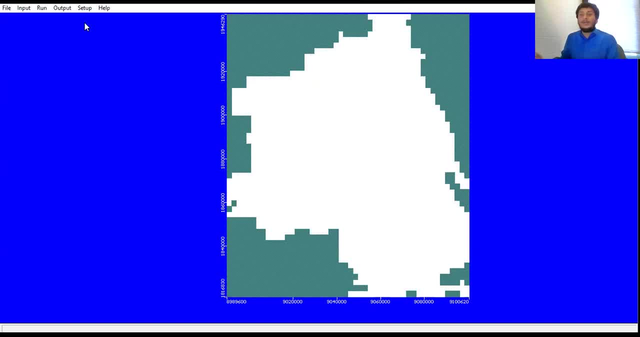 properties to properties, we need to save it. If we don't save because we need to track everywhere, it's kind of it's not very easy to keep on like tracking. we need to track if we don't have any. 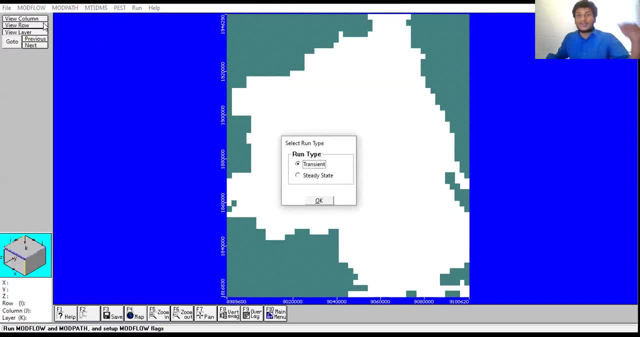 track. we don't know where the error is. so again we have to start from the beginning So we can say we can run the model in transient state or steady state, let's say usually these options we will use to calibrate the model in the. I'll explain the. 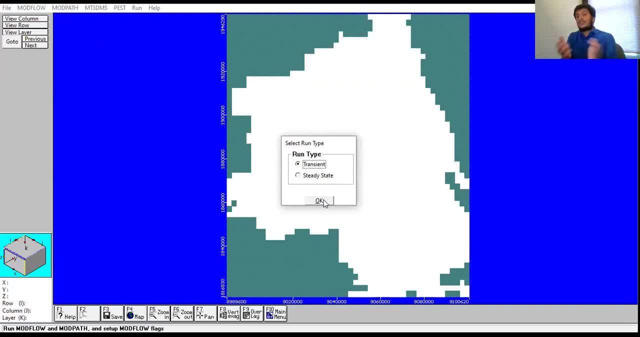 about the calibration and all in the so calibration. So usually if we have 10 years data, if we have 10 years data, so we will say we will use 2-3 years data for the calibration. 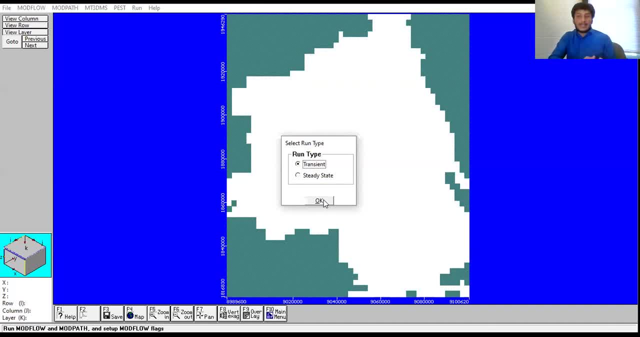 Calibration will tell us that, yes, I created, I recreated or recreated the real conditions in the model. So so what we'll do? we have 10 years data. we'll just use 2 years, 3 years data. 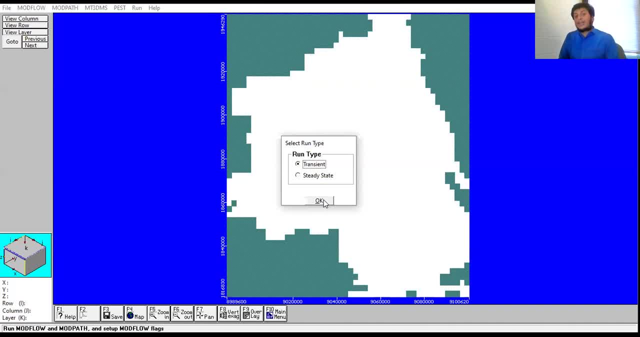 and we'll recreate the model. After creating the model, we'll run the model, we'll get the output. By seeing the outputs- outputs, groundwater levels- we would say yes, it is well calibrated. So it's kind of calibration and validation. Calibration initially we will do in steady state conditions. 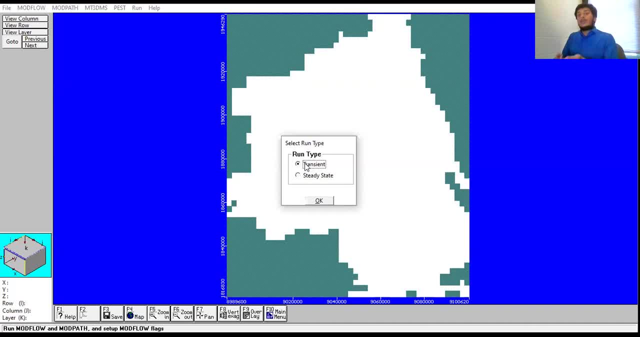 Then if it did well, then we will go to transient state. That is how these options will help us After steady state, because in real conditions obviously there will be transient conditions. so steady state conditions in many cases- I don't say 100%, I cannot generalize it. 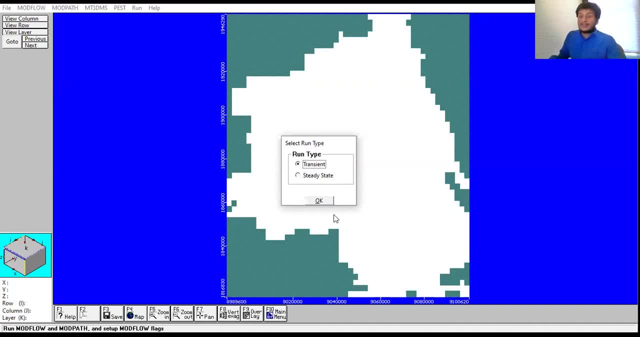 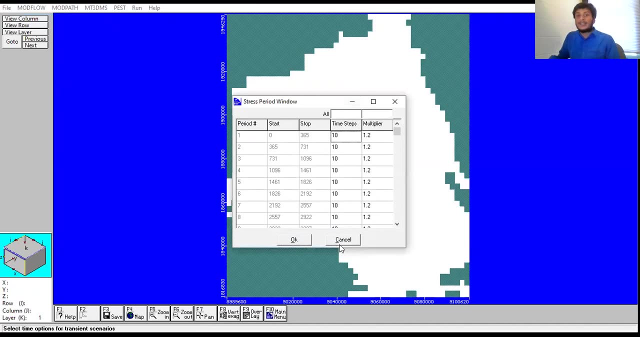 but yeah, most of the cases we'd see transient state Used to generalize. but so so here we have mod flow, time steps, initial heads and all multiplexer- sorry, multiplier. these things will help us to run the model. Just click run If you want zone budget. 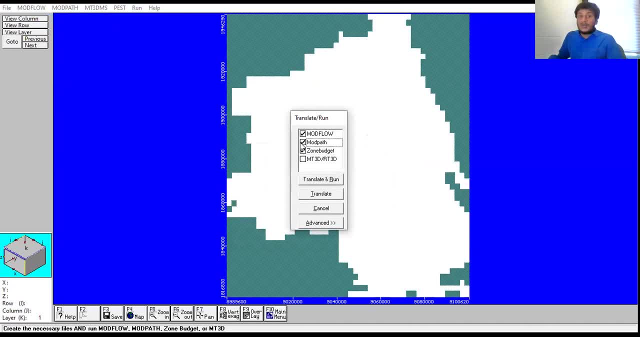 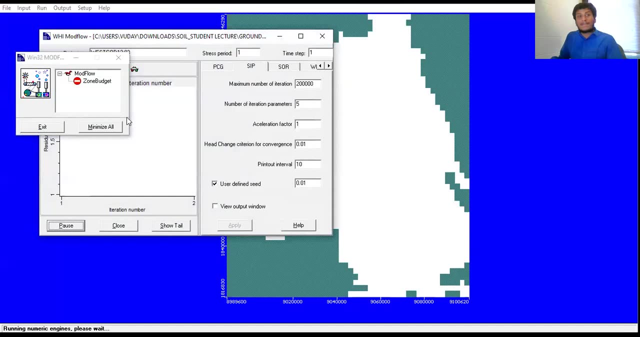 just click it. If you don't want world path, click it. This is for so. so your transport model? Just ignore it. See translate and run. That's all I hope it will run. Let's see what's going on. 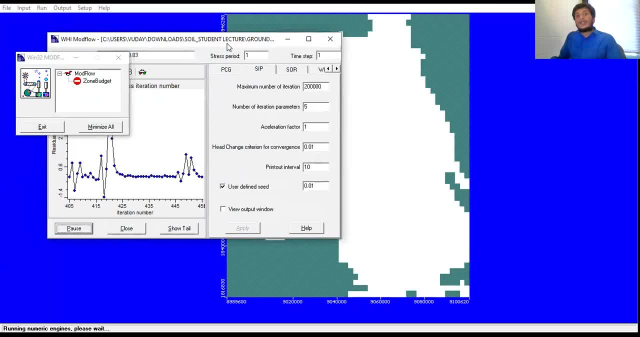 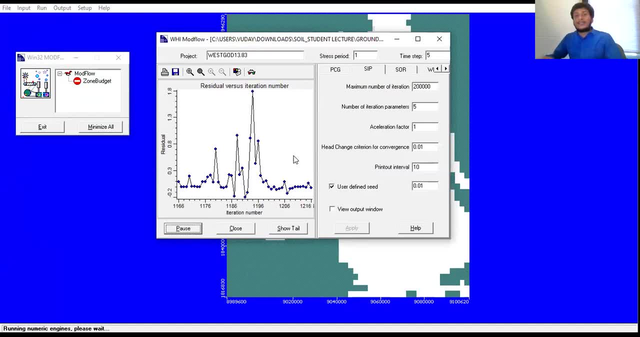 This shows that our model is running. You can see here it's going a little slow. It's actually going so fast, I don't know why. Yeah, let me see, I'll show this So I can just scroll down. maybe I was. 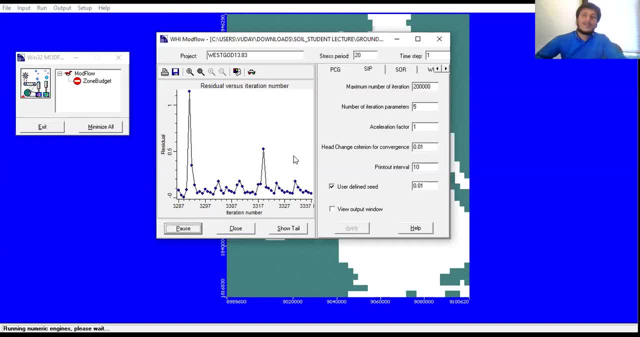 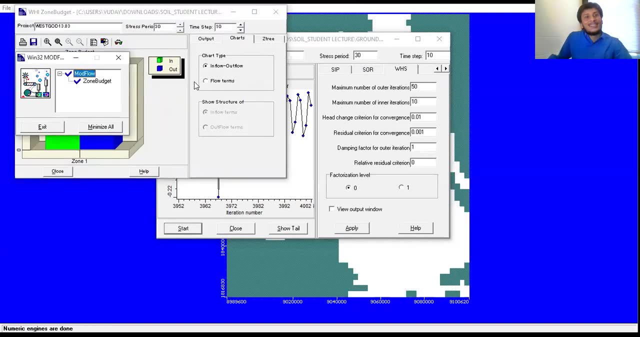 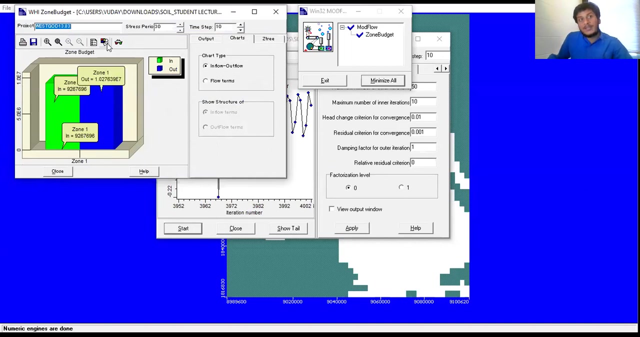 let me just go back one more time and it's going to run smoothly. These are the solvers: PCG, SIP, SOP and WPS. Yeah, we got it. So we got it. You see here. this is the zone budget in and out. this is inflow and outflow. this: 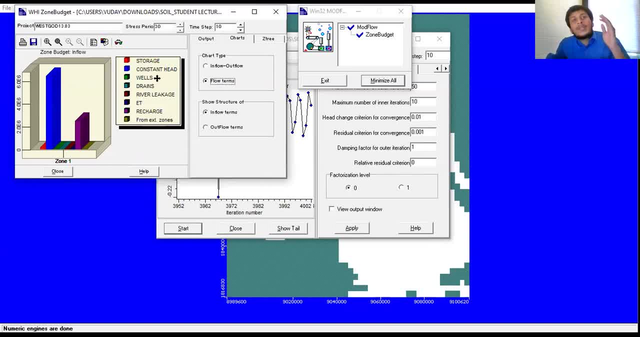 is the flow terms. so inflow terms again. we got some storage. how much we change the view? I guess? yeah, yeah. so this red color represents the storage, blue color represents the constant head, then wells, then drains, then river leakage, evapotranspiration and 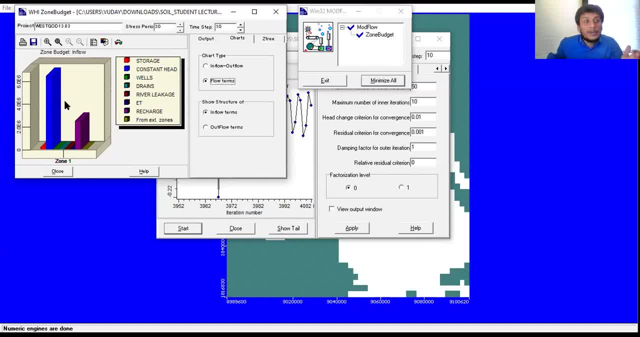 recharge it's contribution, how much? how much like it's contribution. it should say flow terms and it's an outflow. these are inflow: how much water going from our study area? this is the outflow, that's all. we'll close it and we'll open the output ones. 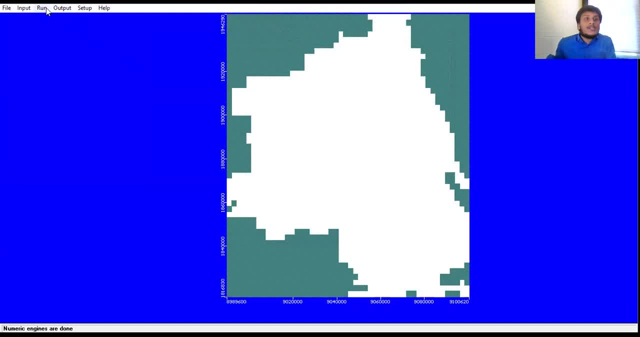 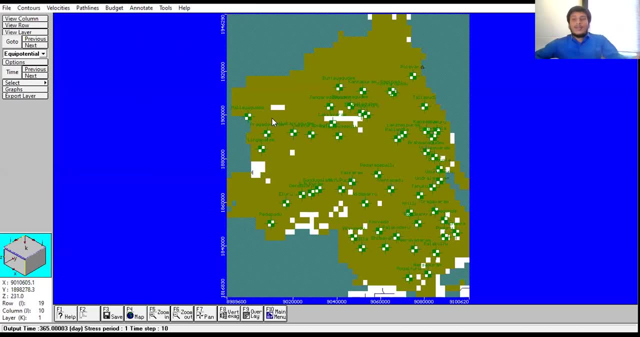 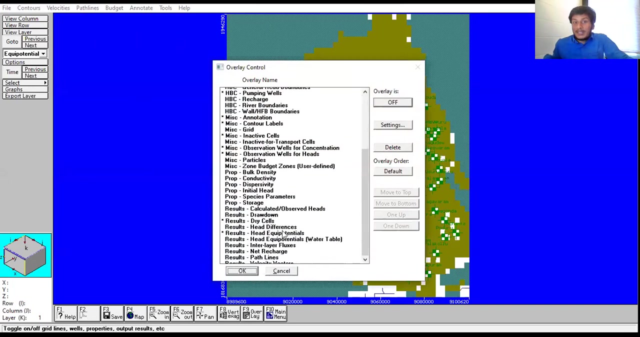 so, coming to the output, I didn't run with the final file. I took some other file. that is why it is showing the dry cell, and my study area output is not like this, though this dry cell. green color represents the dry cell, which means let's see, let's see. 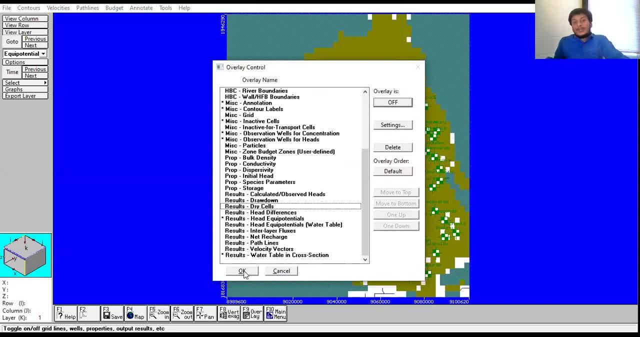 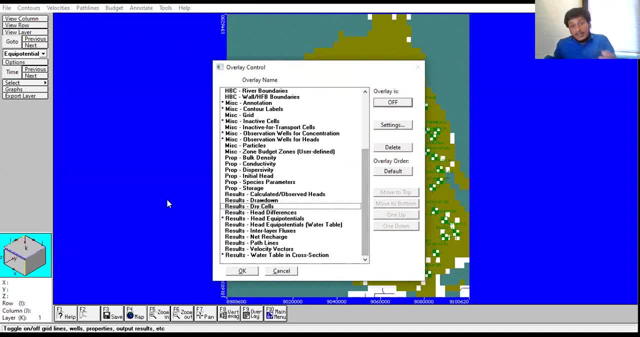 layer. so we have some layers here we can turn. turn them off if you want to see them. we can keep them. if you don't want to see them, just remove them. I'm going to see velocity vectors and other. let's see net recharge and if you want to see some, we. 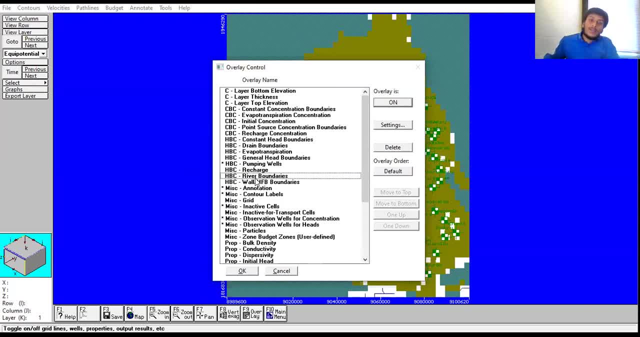 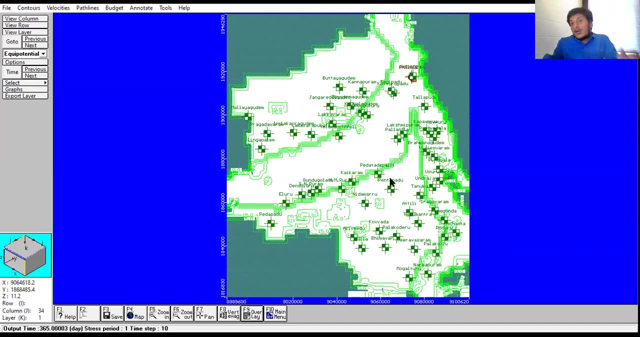 have some other layers here, let's say, annotation, river boundary. if you want to see river boundary, you want to know we can, we can change whatever we want to see. now i remove that. so this is, this is the output. now i would like to see the graphs and to see, to study the layer. i mean i have to study. 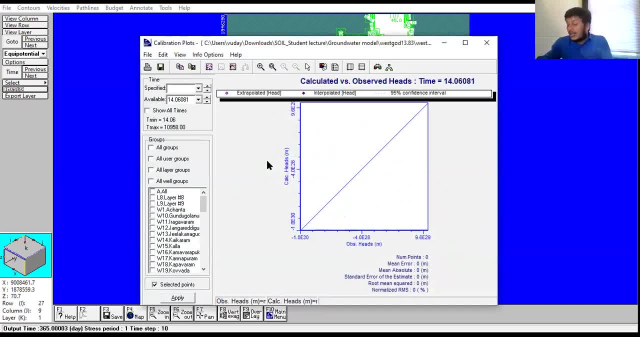 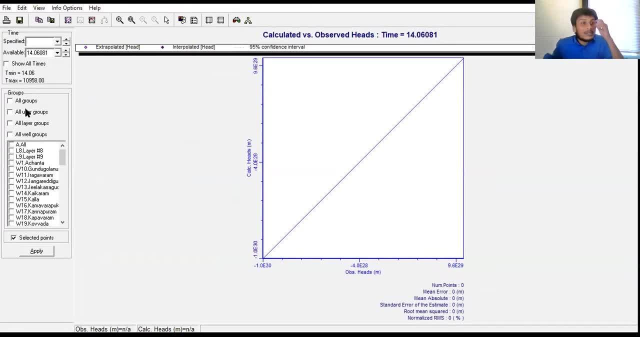 the uh, compare the water level. i have five minutes more to so. yeah, so to see the rms editor. now just see. this is the output. i just click all groups and apply. so when i applied it i got rms 13.84. it should be close to 10- 10.. as close it means our borderless for. 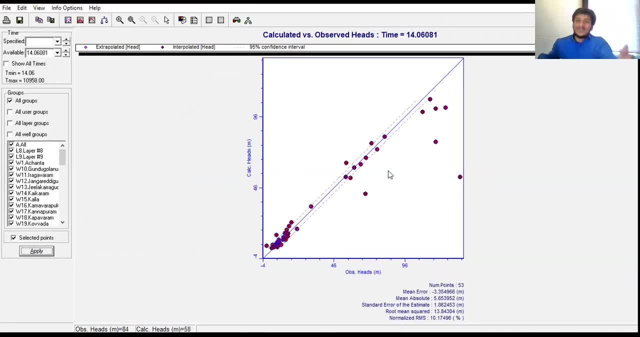 some somewhat fills up almost away from from it, which means they are not well calibrated or or some other error they might be. they might be calibrated, they might those locations they might be. they're having more number of layers. so you can see most of the observational came very close to 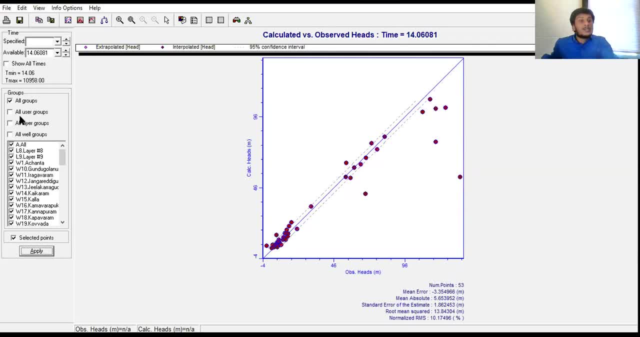 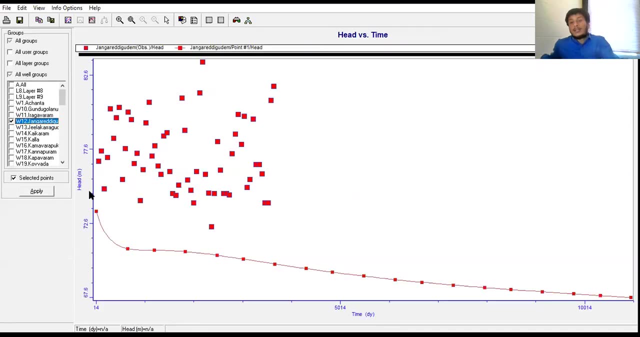 the line. so i would like to see the output. suppose, select a and we got it selected like this, just click it. this shows the actual scenario in the groundwater. so in the in day, 14 groundwater level is here in. slowly it's coming down, down, down down. 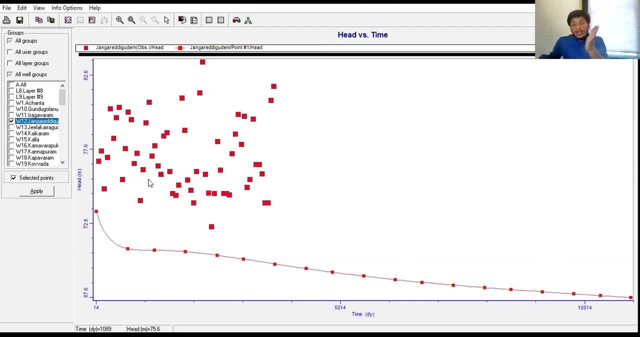 it's moving like this, it means groundwater will keep on going. this is completely accurate. this is the first time this is happening in all water bodies. this is the first time this is happening in all water bodies. it is away from all water bodies. it is away from the canal. it is away from. 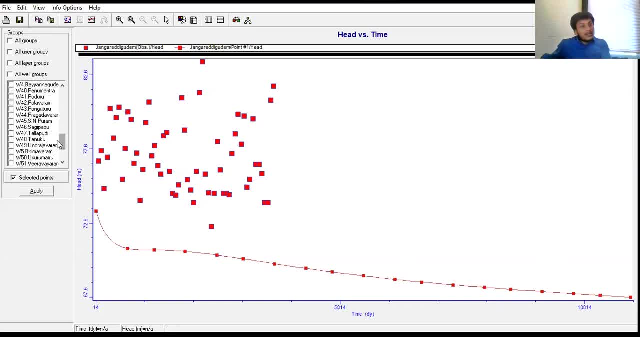 the river. it is away from the sea in my study area. let's see some other. if you, if we see this, it initially go ahead is there and it's it's ongoing. this is little here, because in this day, like from this, like one year before, like almost six, six months before, 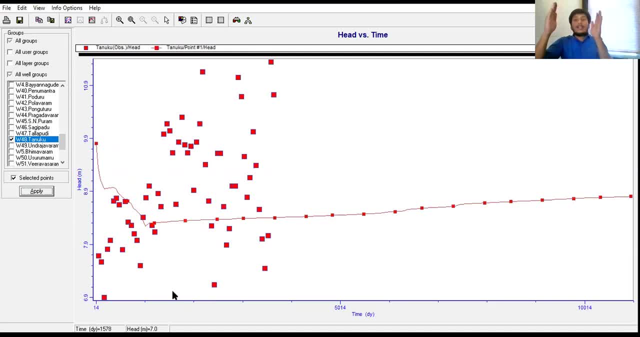 water started flowing through, like, as i mentioned earlier, we have river a godavari river, river b krishna. so krishna river doesn't have enough water, so they constructed an irrigation project to uplift the water from river a to river b, river godavari. so this village, or this observational 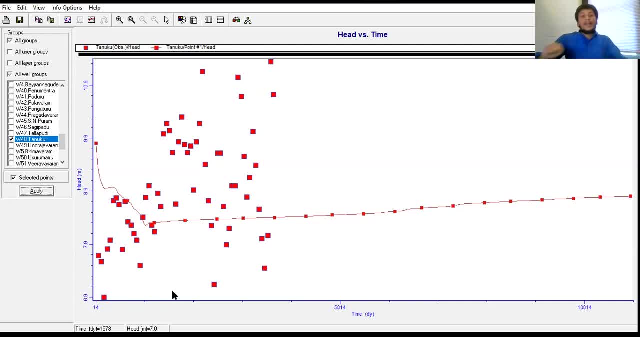 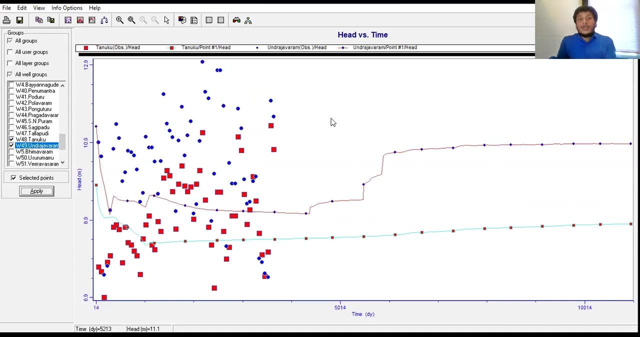 is very close to the interlinked canal, so that is why, opposite it is, you can see the rise in groundwater level. that is how it works. if you want to see, if you want to see two, three wells together, this is how this is, that is how it looks, so you can see. this is the uh, which is uh. 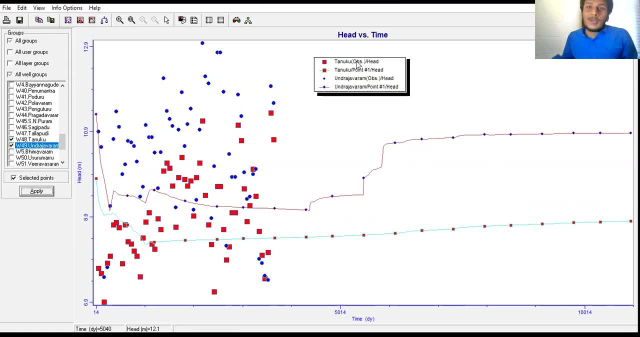 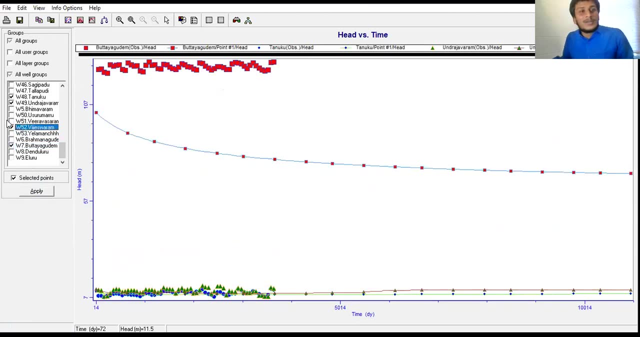 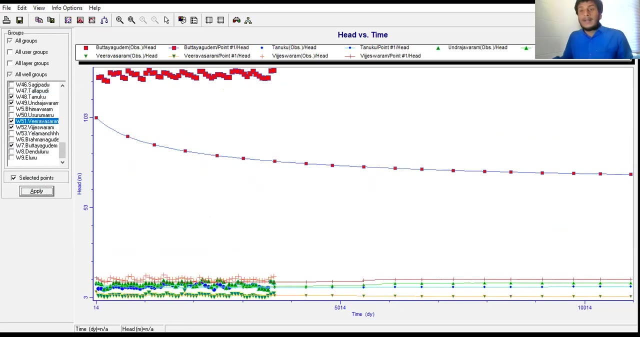 the location of another observation. well, which is a location of another observation? well, so this is a water observation. we can say, like we can see many observations, the water, whatever diagram, these are names of the observations. yeah, which is from vr? yeah, you can see, these are like: this is this. that is how it works, so let me close this. 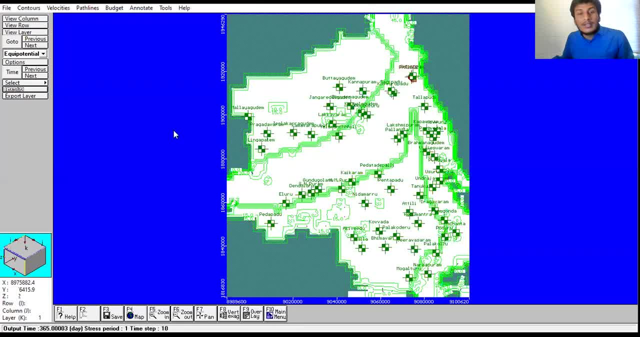 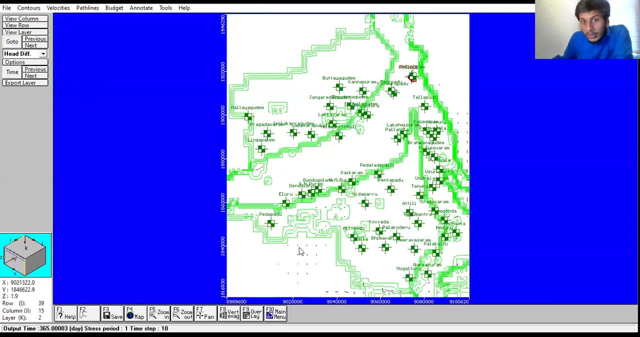 i think i can't close this now. yeah, when i when i started to uh strange money. it's not allowing me to close or maximize or minimize the scale, you know. uh, i am done with this. then go to head differential, more like how much difference you can see the contour contours. 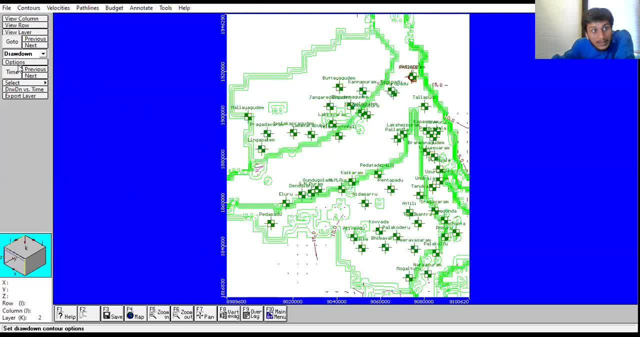 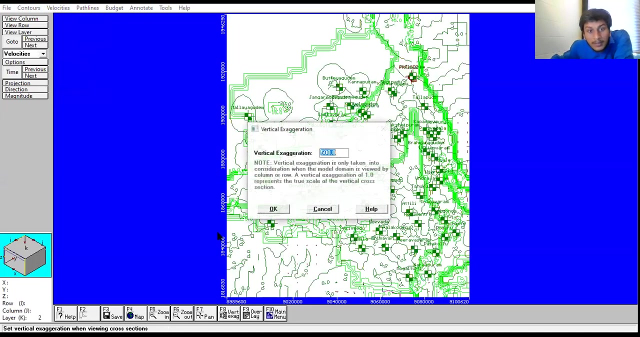 these are the velocity vectors. let me explain them. this is the drawdown curves, contours and all like how water flowing flows show you one thing: you can see the high plugs in the study area say let me zoom it- exaggeration. you can see the water flow if, if, if. 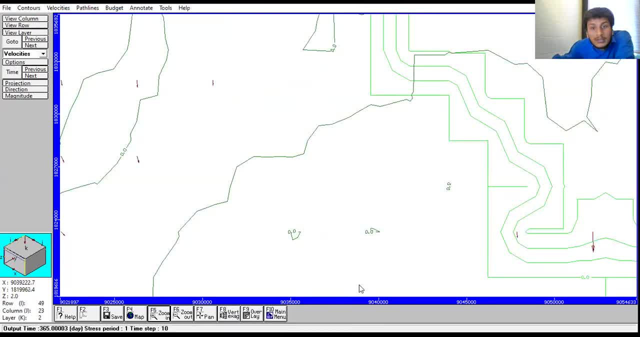 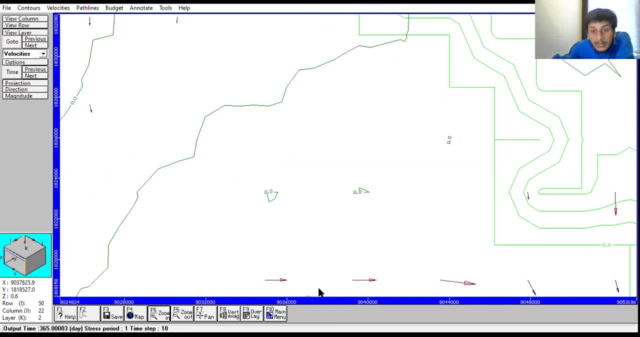 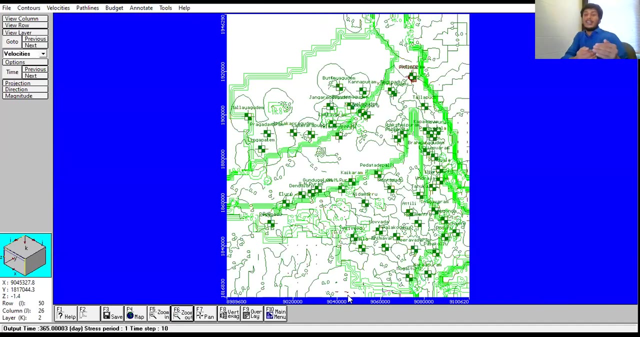 you can see the arrow marks here, right? i hope you guys are able to see this. yeah, this shows the water flow direction. this is like: uh, let me, yeah, so you can see, this water is flowing away from, away from the study area, and it's going towards the sea. towards the sea, which means it means. 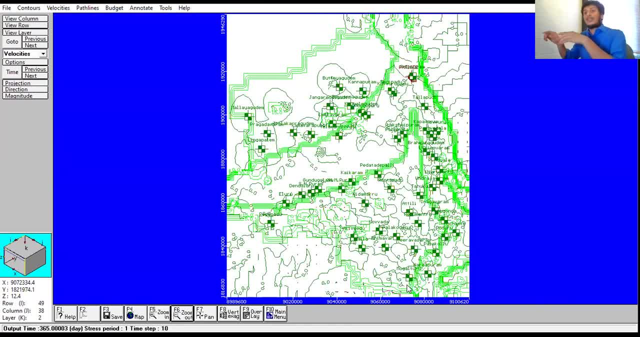 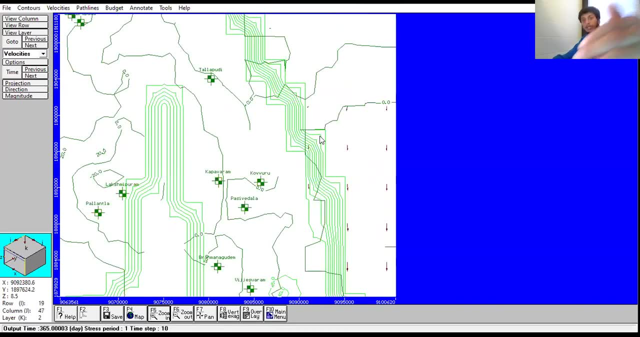 obviously, water will flow from high elevation to low elevation. that's what happened there. it is representing that you can see when you, when you zoom in this location, you can see the water flow. water is flowing towards the sea and coming towards the river. this is the river location it's coming. 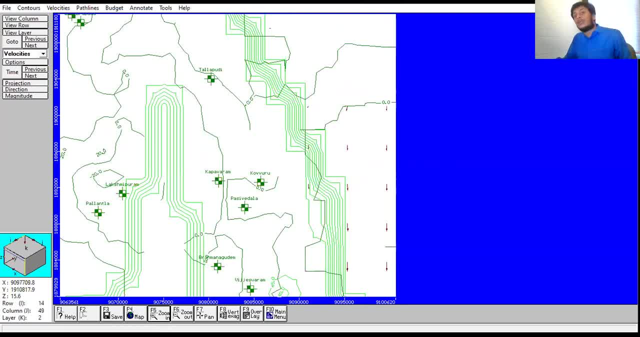 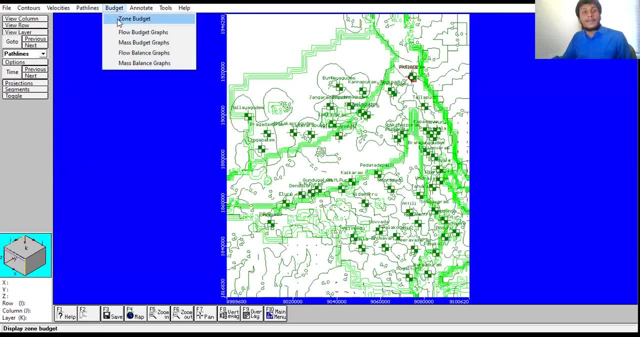 towards the river. it's coming towards the river together, going towards the sea. that's what it's doing. then we are going to see the budgeting. some other outputs are there. i, i should, i, i don't have enough time, i guess- zone budget, zone budget: zone output. you can see the numericals: how much water, how much river leakage? 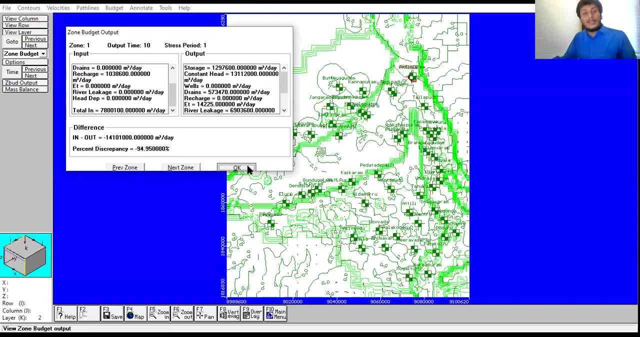 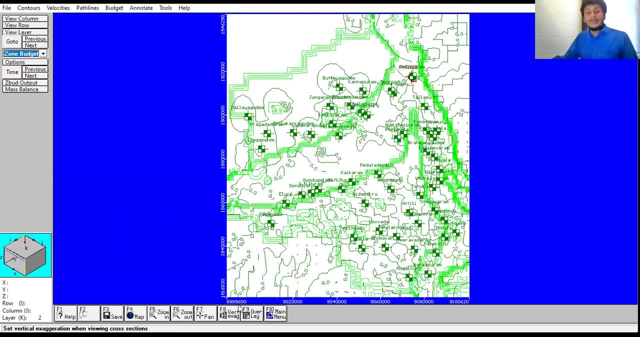 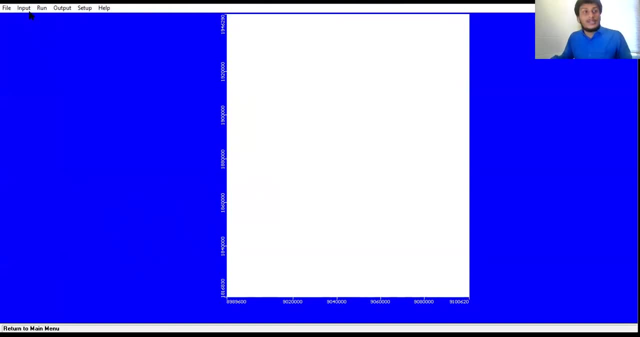 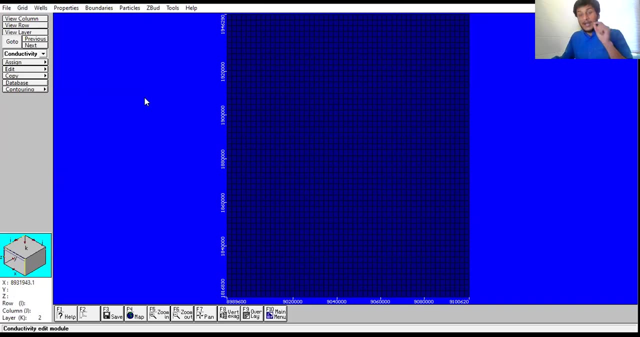 how much the the graph which we saw there can be. i'm sure i think, yeah, that that's how it works. i think just a moment, like within a two minute, within two minutes, i'll try to show the layers. i forgot to show you that, so go to the uh properties: conductivity. 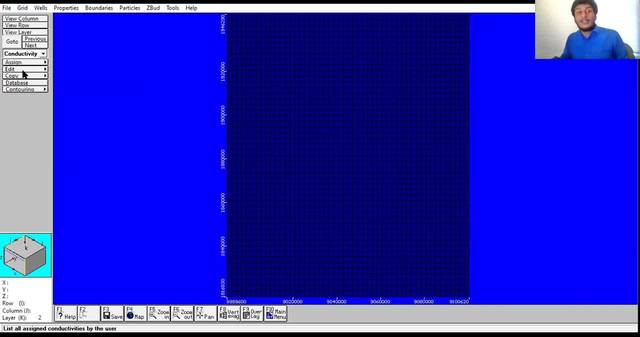 how i assigned the conductivity. i said, but i didn't show my uh, show the yes, right, let me show it view column. view column will help us to see. so this is the, this is how our soil will be, but we? this blue shape is the top surface. 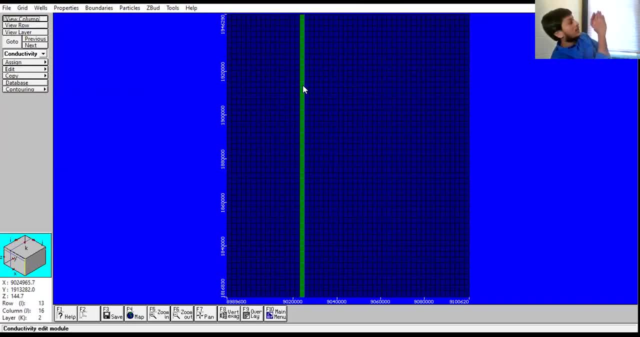 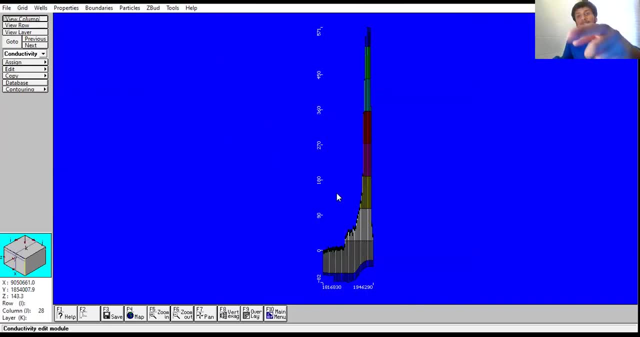 soil surface. this is, this is. it's what this is what it's showing. so, if we want to see the layers from the side, if we want to see the layers from the side, this is how it looks. who close them? make it 500, exaggeration, zoom out a little zoom. 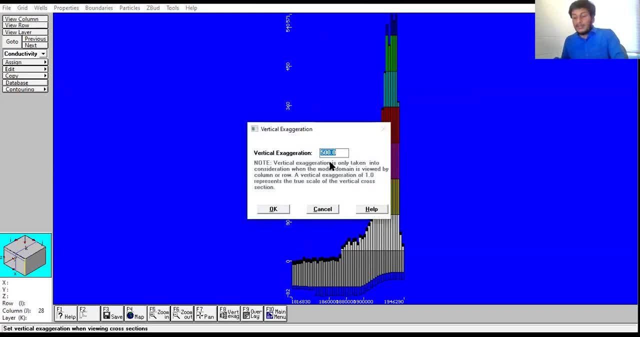 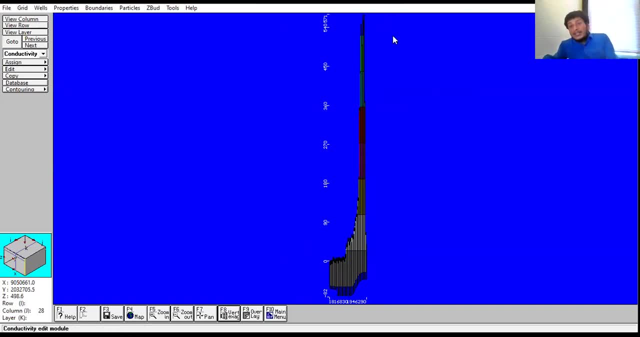 we. we need to make it some 1500. you can see that it's going to show that this is because in some location it has the highest elevation point in my study area. that is how it looks, and let me view through the row, let me view through column. 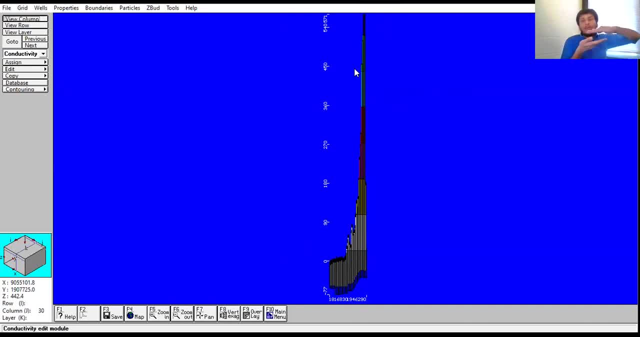 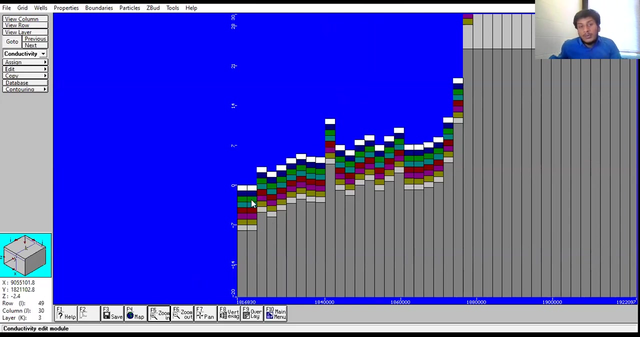 so this shows. uh, so this is the column view, this is the row view, this direction i'm seeing it, row column. that is how, like we are, we are seeing all the way, all the way you can see. so if we zoom it, to zoom it here, so we can see the top layer, blue, three, four, five, six, seven, eight, nine, nine layers. 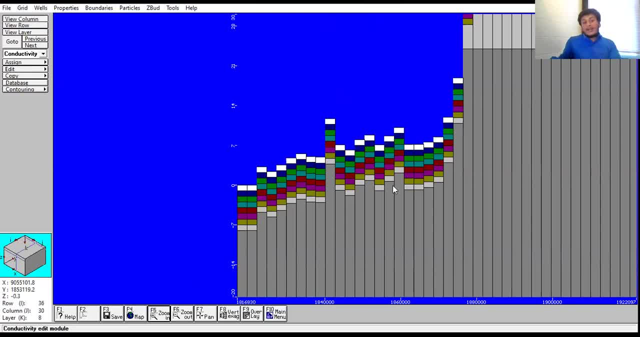 in one location. we have template. that is how i created the model. this is the sanctions. this is a little complicated area so we got too many areas, which is kind of headache. so we are going to give conductivity of each location. i'll try to show you that. let's click. 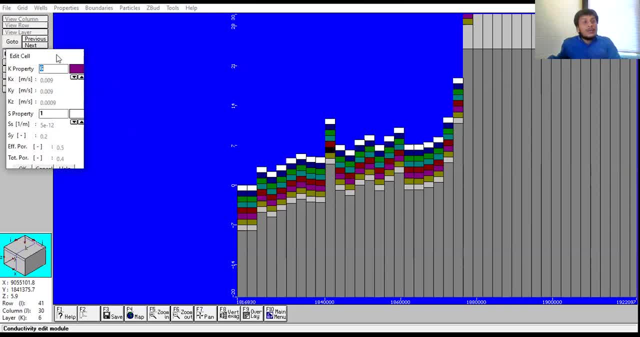 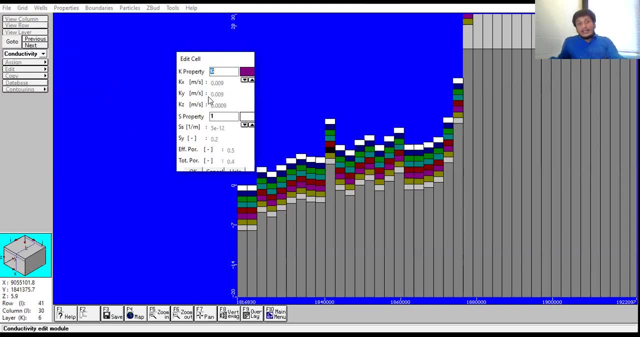 here. so if we see here we'd say property number, layer number is like sorry, layer number is six, i guess, yeah, it's kx k minimum ky kz z is like almost 10 percent, yeah, 10, i guess, yeah, 10 of the kx and y.